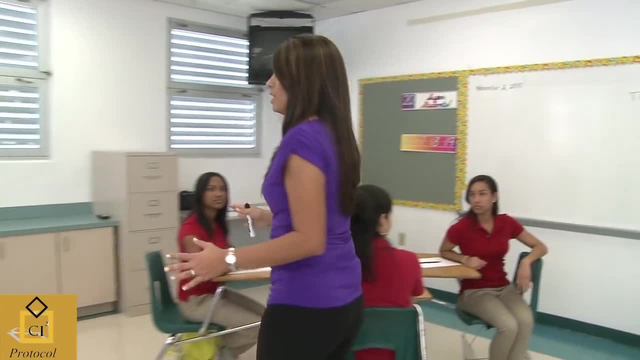 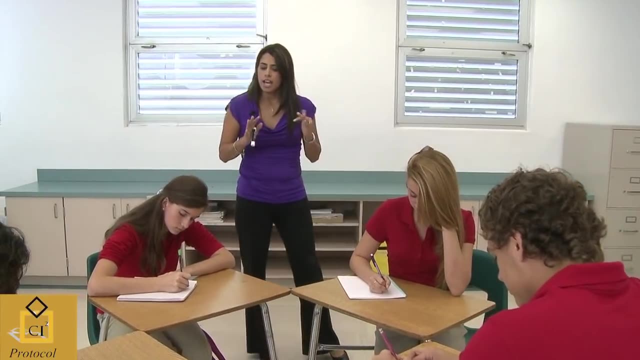 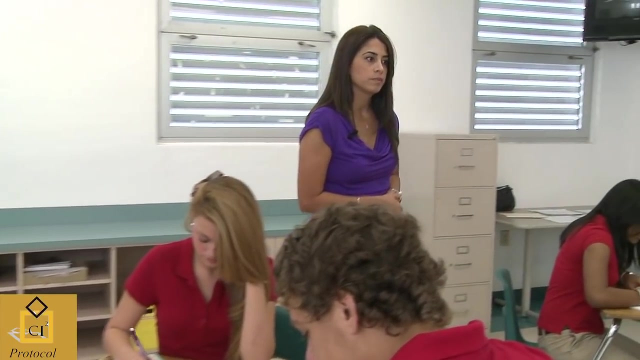 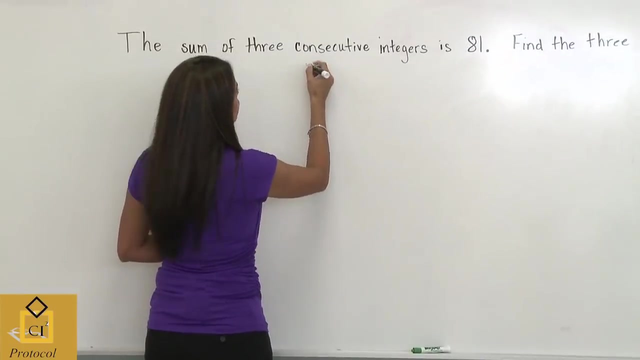 I want you to attempt this problem any way. you want to attempt it. Take a couple of minutes, write it on your paper, try to figure it out and we're going to see if we have different approaches to answering this question. Before we begin, I want you to take a really close look at this word. 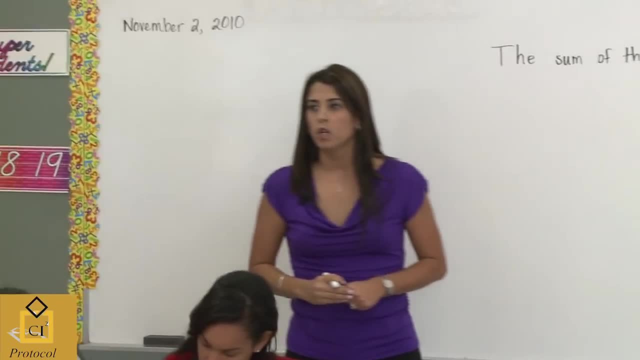 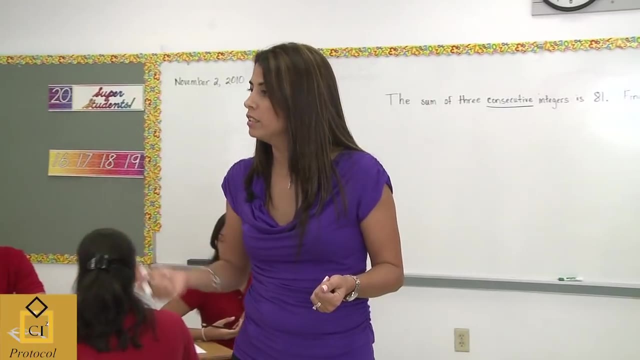 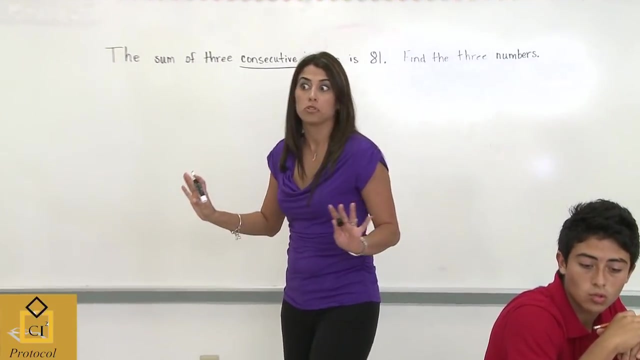 right here: consecutive. What does the word consecutive mean? What does it mean to you? Give me an example, if that's the way it's easier for you to explain, Like one after the other, One after the other. Okay, so give me an example of three consecutive numbers. 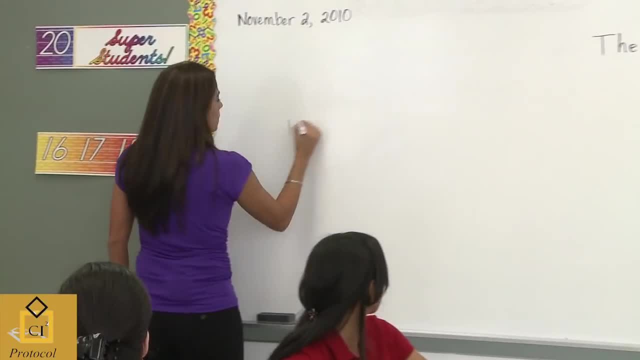 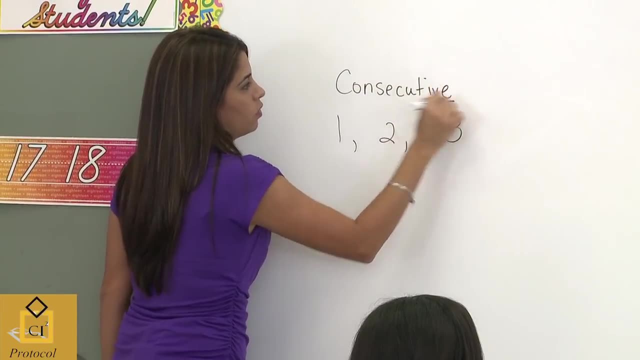 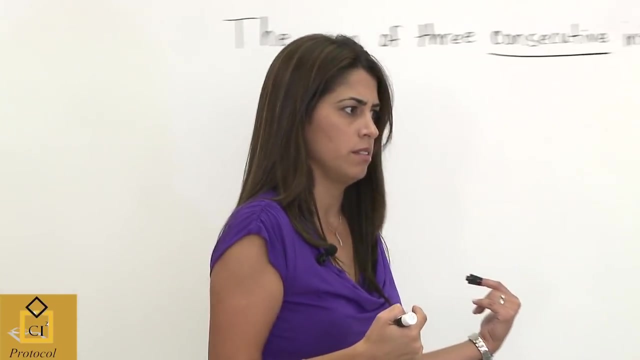 One, two, three. One, two, three, Okay, One after the other. One, two, three. Are those the only consecutive numbers that exist? No, No, No, Infinite, Infinite consecutive numbers. Now give me an example. 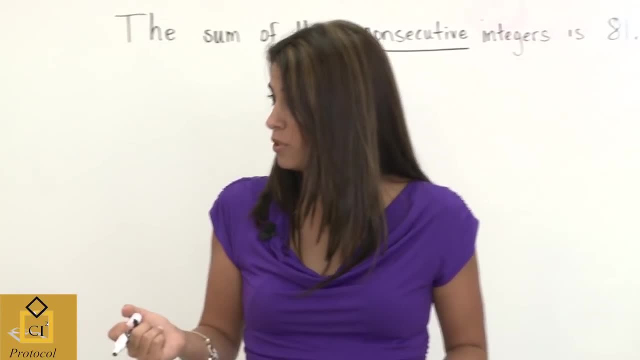 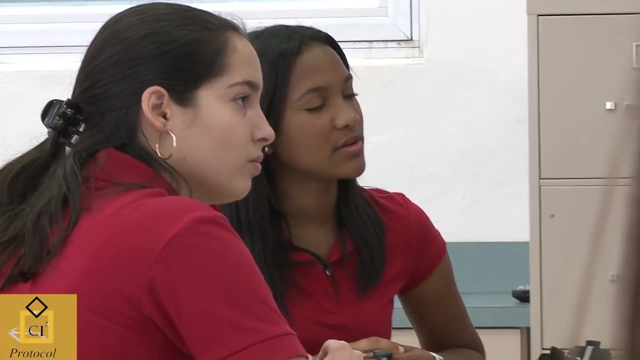 Chris Nell of non-consecutive numbers. Let's say seven, nine and ten. Seven, nine and ten. They're not consecutive. Maybe these two are. They're not seven and nine. They're not seven and nine, Okay. 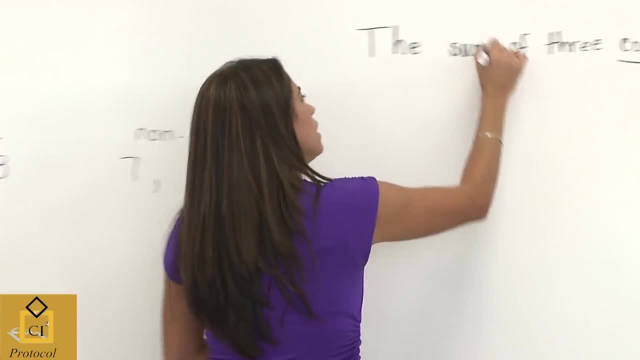 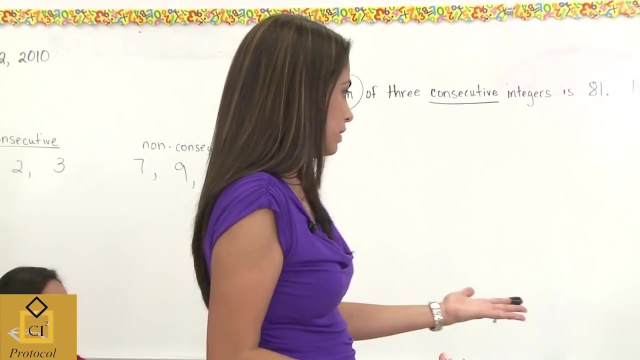 Okay, let's look at one more word in this lesson: Sum Hector. what does sum mean to you? It's the addition when you put them together. When you put them together, Fantastic. So it basically means addition when you put them together. 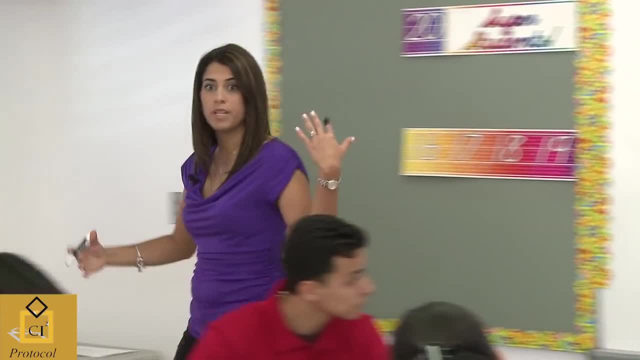 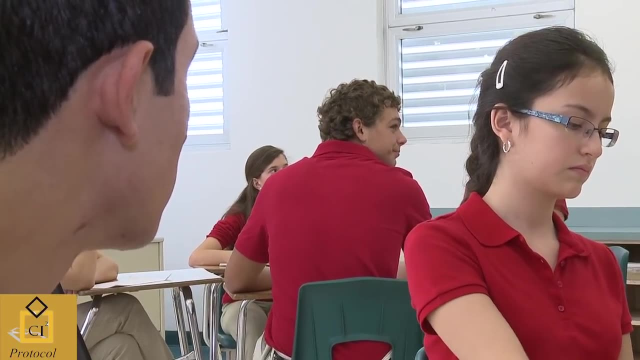 Okay, so now let's read the sentence. Chris, can you read that sentence for me again, See if it makes a little more sense? The sum of three consecutive integers is 81.. Find the three numbers. Okay, Annabella, we're finding three numbers. that are what? 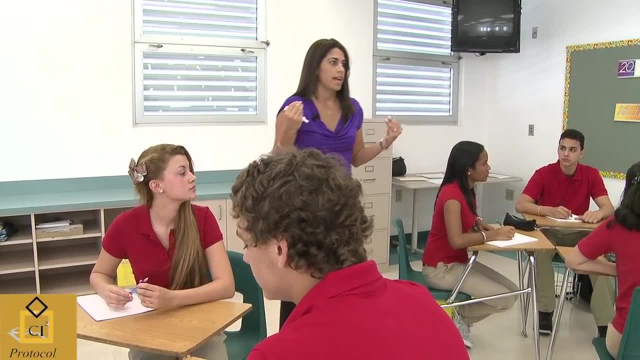 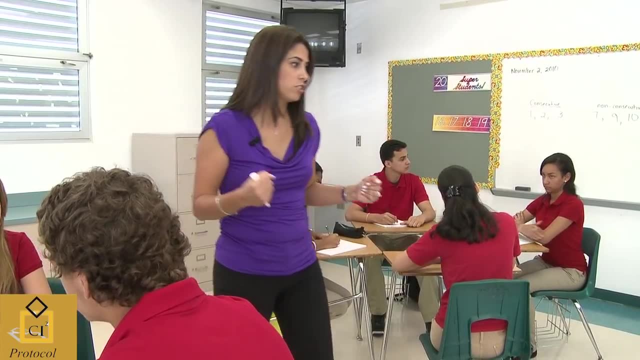 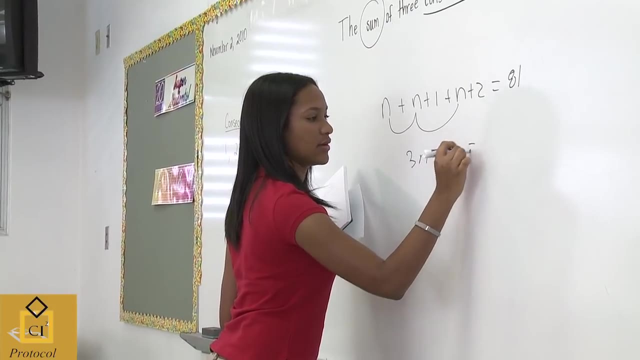 Seven That are next to each other, Next to each other And Daniela, whose sum is what? Eighty-one, Eighty-one, Okay, now attempt the problem. We have a clear understanding. I believe Having whole class discussions of student solution strategies not only builds a community of learners. 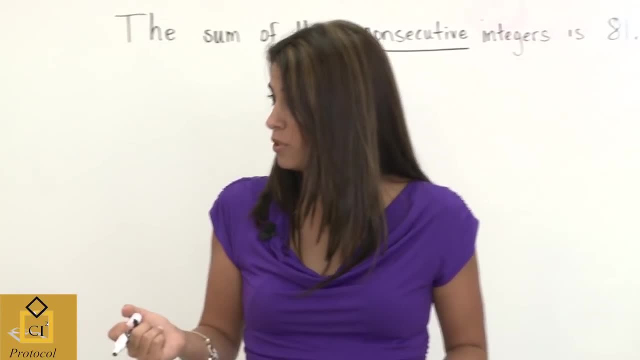 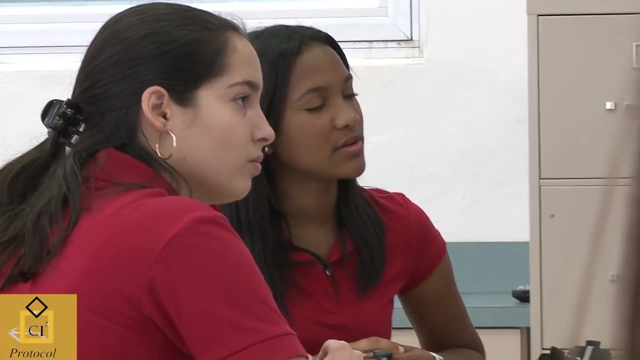 Chris Nell of non-consecutive numbers. Let's say seven, nine and ten. Seven, nine and ten. They're not consecutive. Maybe these two are. They're not seven and nine. They're not seven and nine, Okay. 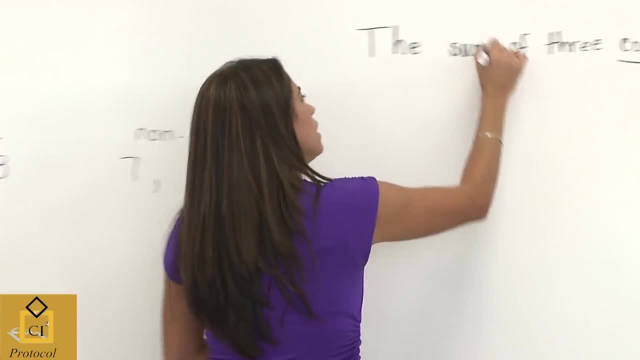 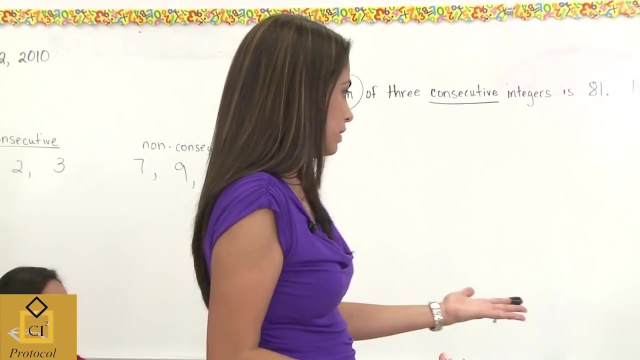 Okay, let's look at one more word in this lesson: Sum Hector. what does sum mean to you? It's the addition when you put them together. When you put them together, Fantastic. So it basically means addition when you put them together. 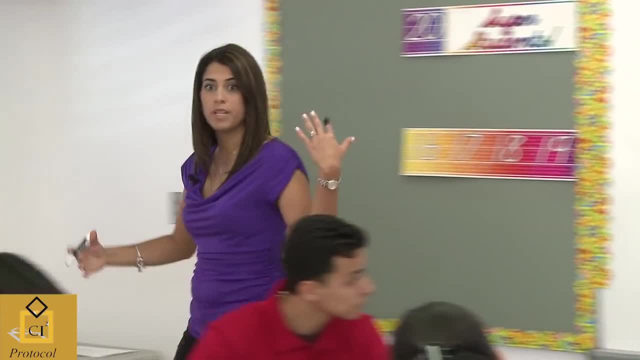 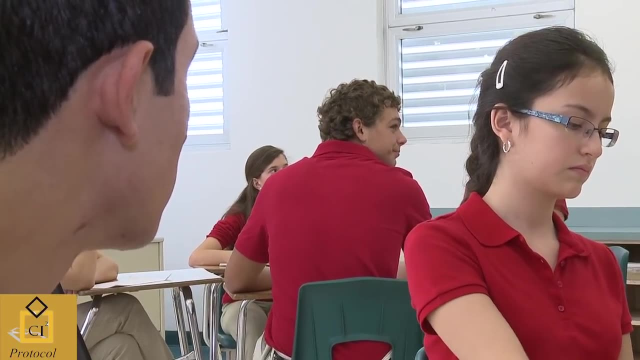 Okay, so now let's read the sentence. Chris, can you read that sentence for me again, See if it makes a little more sense? The sum of three consecutive integers is 81.. Find the three numbers. Okay, Annabella, we're finding three numbers. that are what? 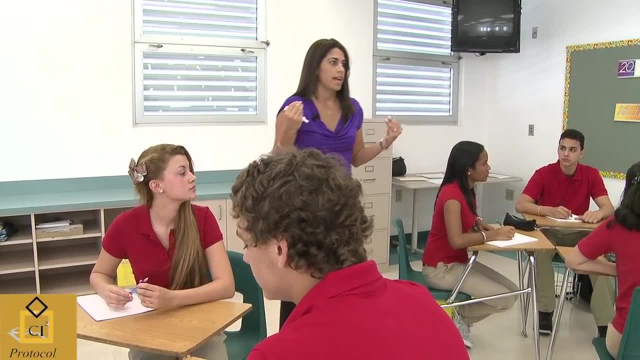 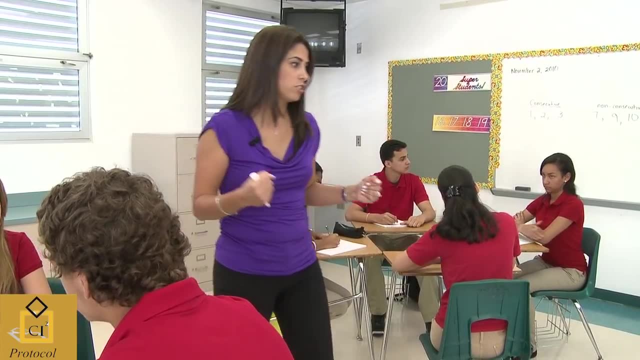 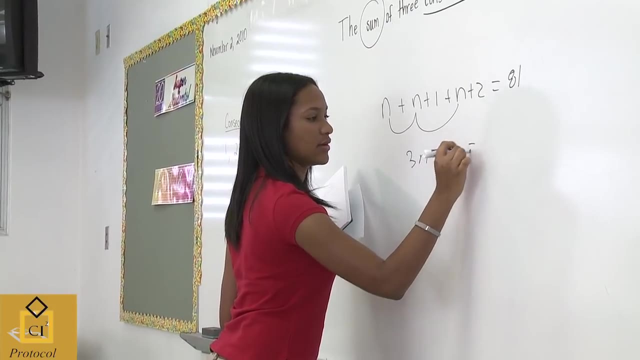 Seven That are next to each other, Next to each other And Daniela, whose sum is what? Eighty-one, Eighty-one, Okay, now attempt the problem. We have a clear understanding. I believe Having whole class discussions of student solution strategies not only builds a community of learners. 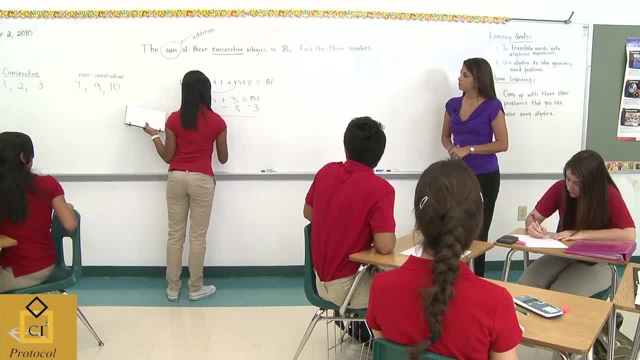 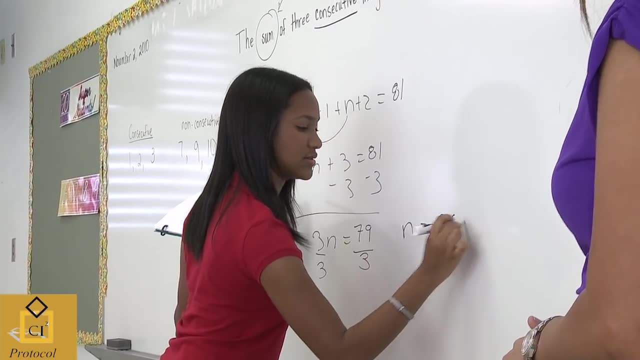 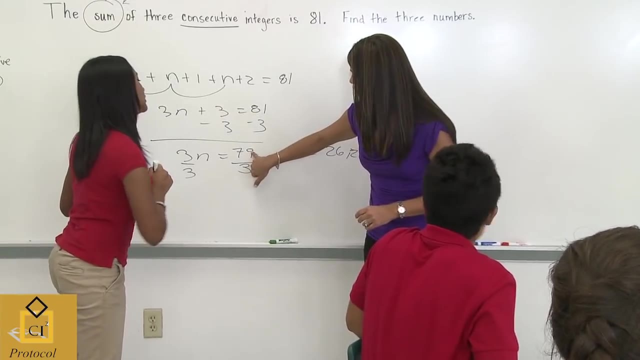 but allows students to see, hear and understand multiple approaches to solving the same problems. This in turn helps to build relational understanding, leading to greater student achievement. Presenting students with challenging, open-ended problems, then having them defend their work solutions will result in students learning associated skills and concepts at a deeper level. 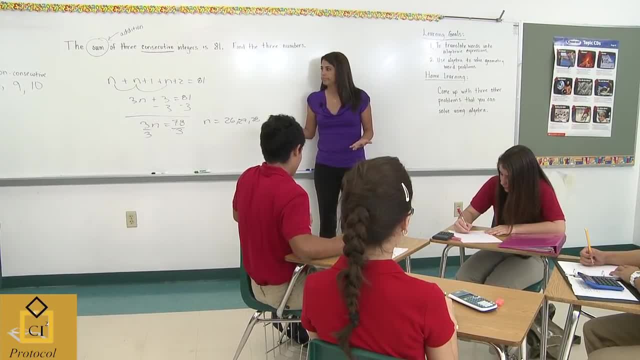 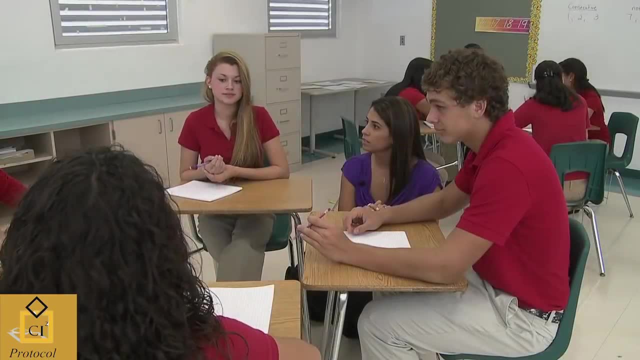 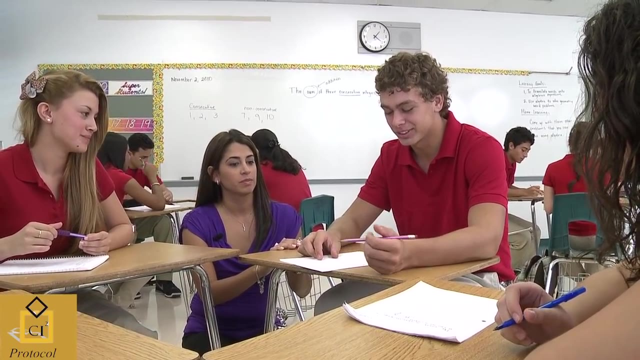 than if they are simply asked to recite factual knowledge or to apply procedures in a mechanical way to problems that have a single correct answer. I did it the harder way. I just. I kept adding three numbers until I got something that equaled to one. 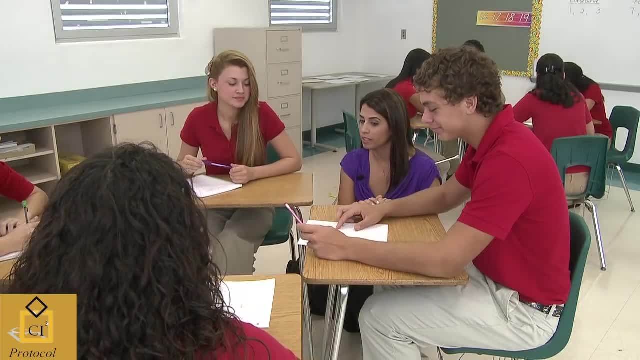 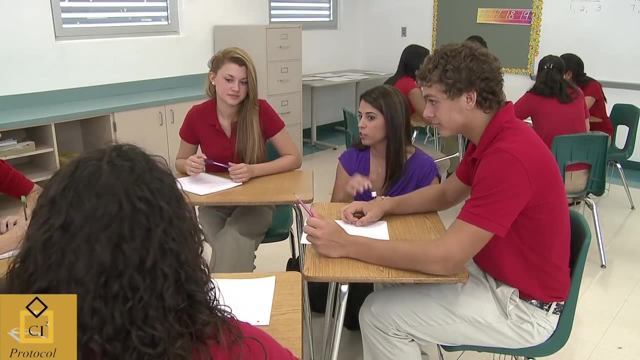 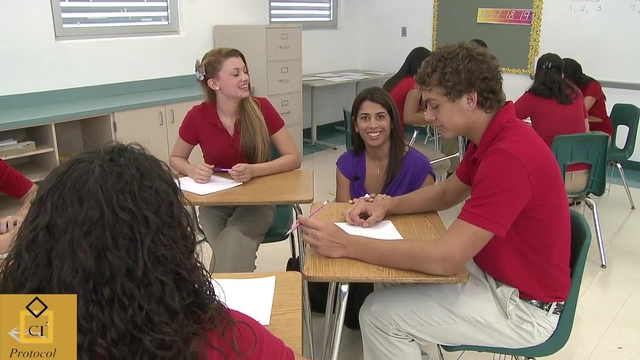 I realized it was twenty, But you still got it and it's very interesting because that's the way it makes sense in your mind- How many of you would have taken her approach. You took it. Did anybody take it? algebraically, Nobody Interesting, Okay. 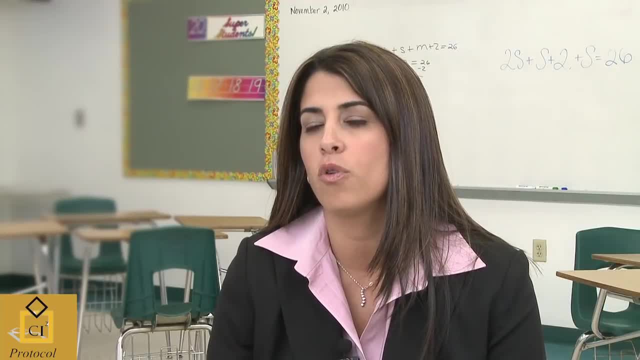 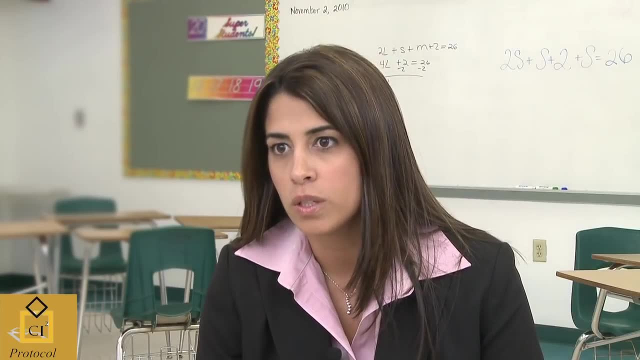 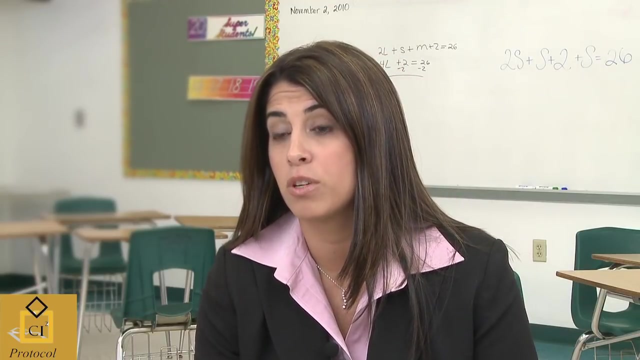 Some students just use, as one student had said before, common sense And they just use a division operation to be able to solve it When another group solved it algebraically, using variables And another group solved it in their own way but were able to justify how they got the answer. 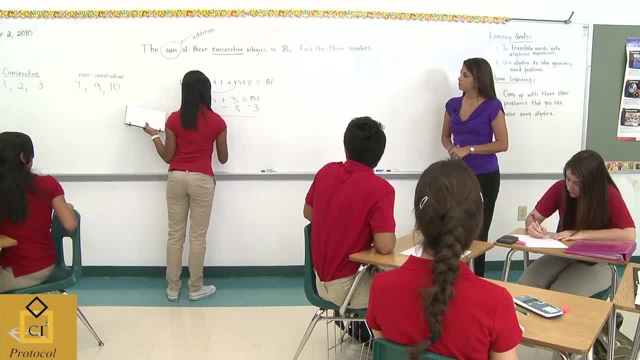 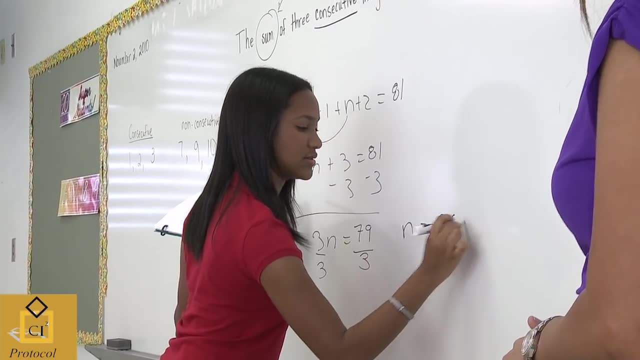 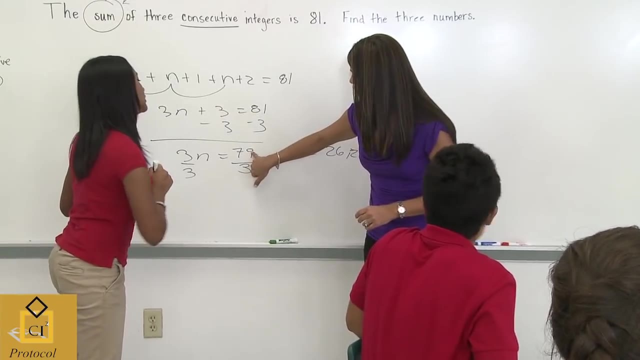 but allows students to see, hear and understand multiple approaches to solving the same problems. This in turn helps to build relational understanding, leading to greater student achievement. Presenting students with challenging, open-ended problems, then having them defend their work solutions will result in students learning associated skills and concepts at a deeper level. 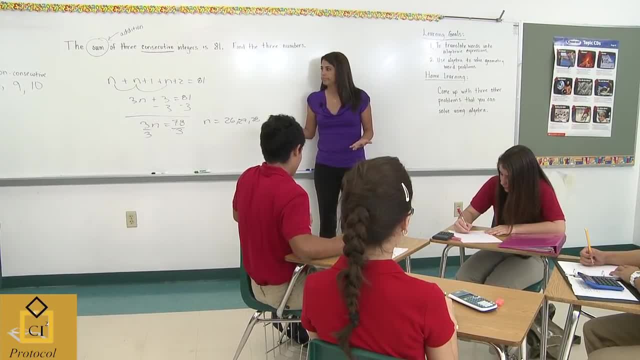 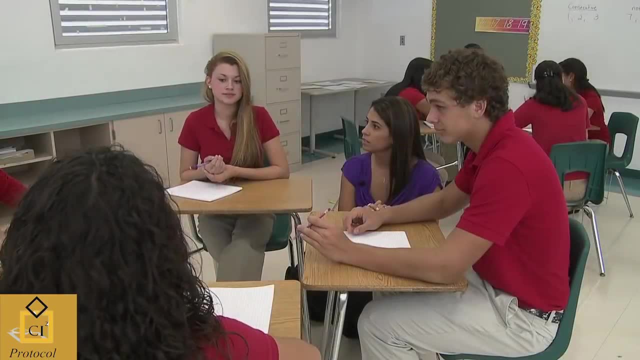 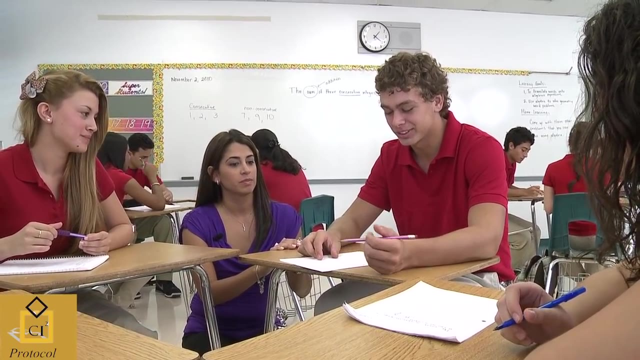 than if they are simply asked to recite factual knowledge or to apply procedures in a mechanical way to problems that have a single correct answer. I did it the harder way. I just. I kept adding three numbers until I got something that equaled to one. 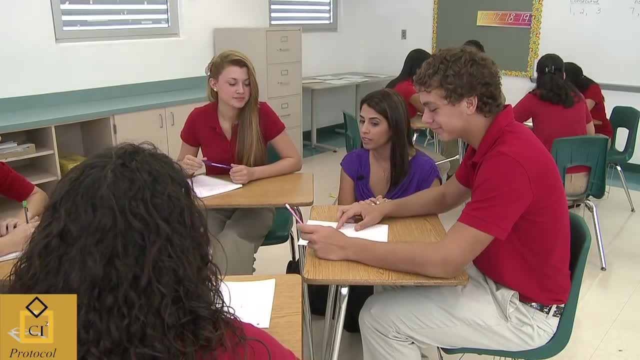 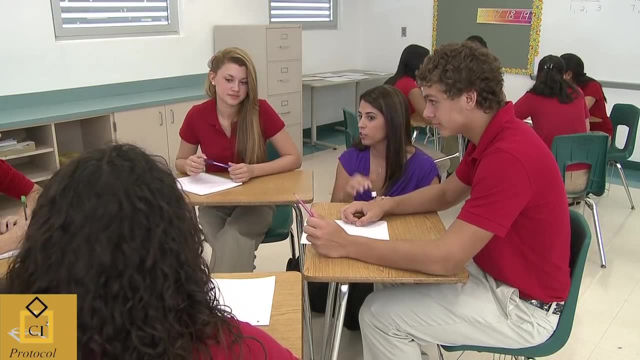 I realized it was twenty, But you still got it and it's very interesting because that's the way it makes sense in your mind- How many of you would have taken her approach. I took it, You took it. Did anybody take it algebraically? 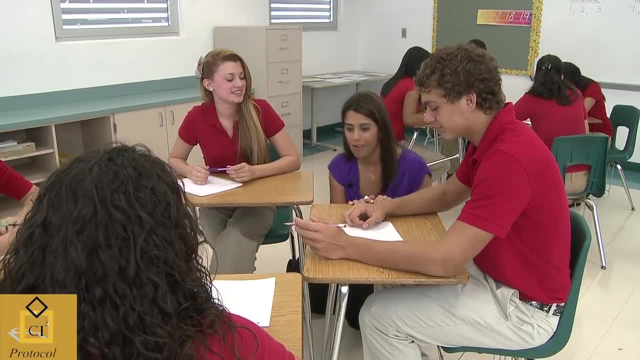 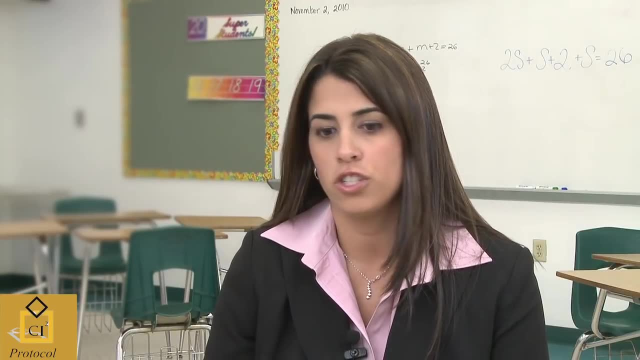 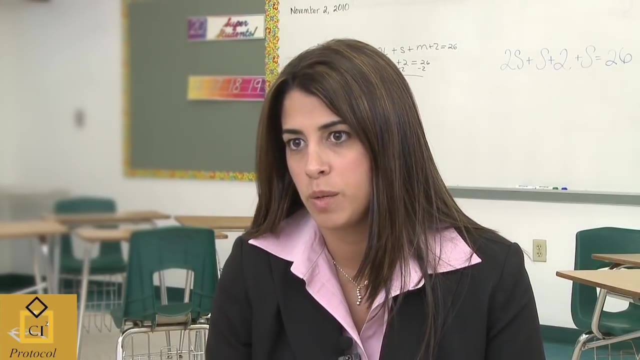 No, Nobody Interesting. Okay, Some students just used, as one student had said before, common sense And they just used division operation to be able to solve it When another group solved it algebraically using variables And another group solved it in their own way but were able to justify how they got the answer. 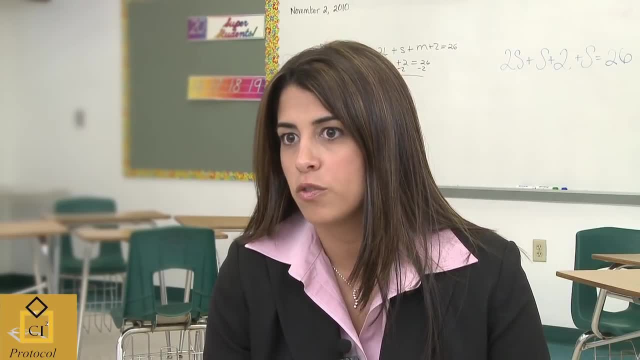 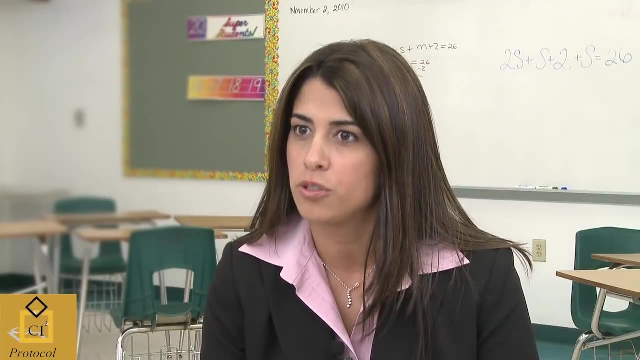 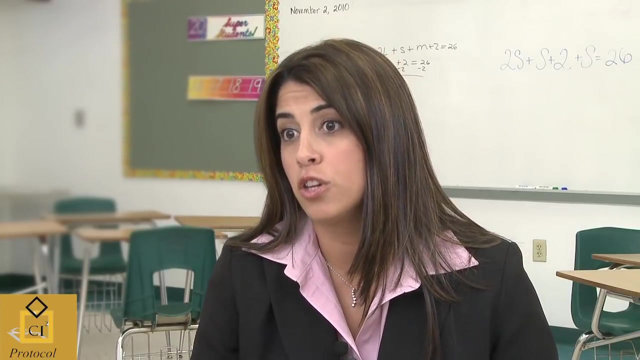 So my main focus, my lesson objective, was to teach them how to translate words into algebraic expressions. So one group had a very clear understanding of how to do that, So I went ahead and worked off them. I brought the students up to the board and allowed them the opportunity, though, to explain their methods. 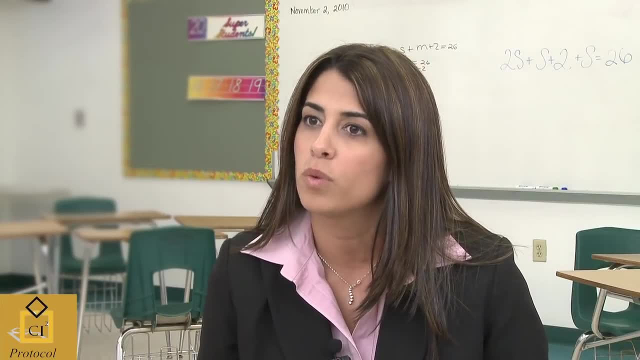 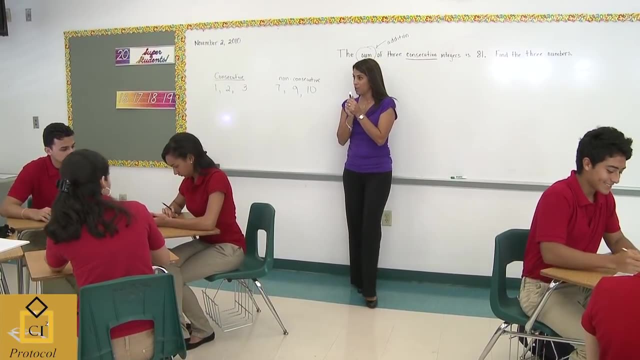 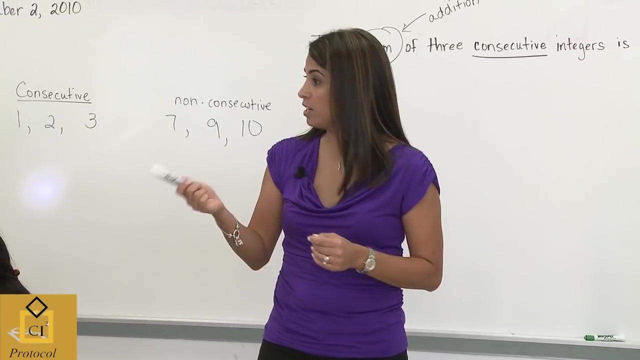 I wanted to show them that there's definitely many different ways to answer a problem And for them to share their perspective on the problem, The ways you got these problems, Believe it or not, every single group did it a little different. Okay, So I'm going to start over here. 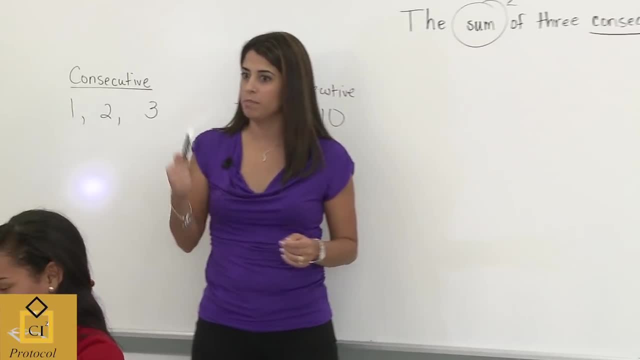 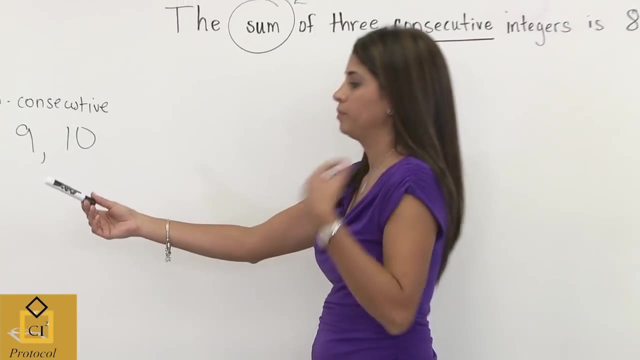 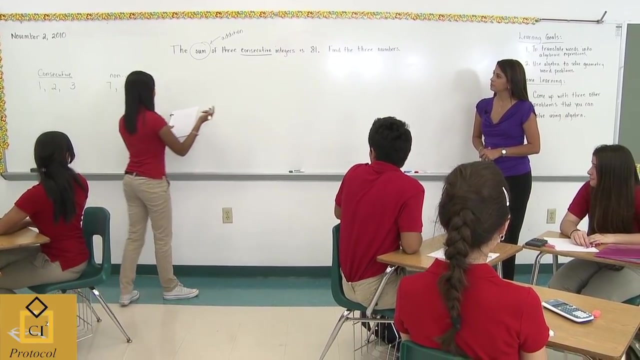 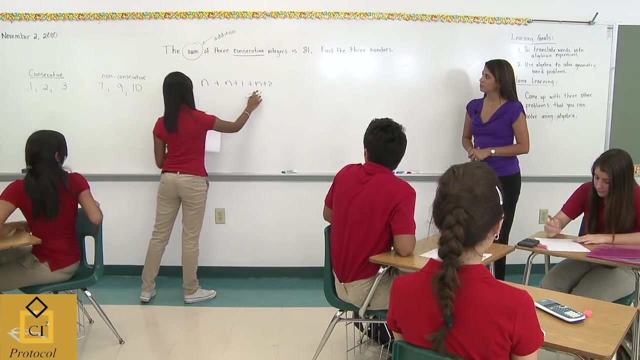 Please pick somebody to represent your group And come on up to show me. All right, Chris, now it's you. I got the answer because it's the same number, so I use a variable- It's n plus n plus 1 plus n plus 2, because you're finding three different numbers. 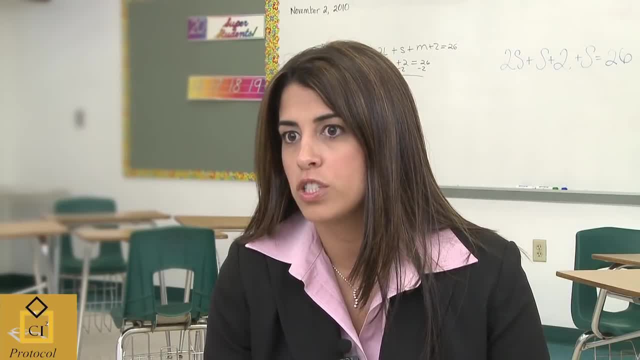 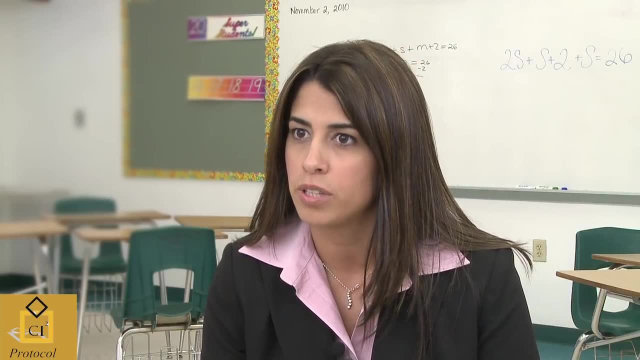 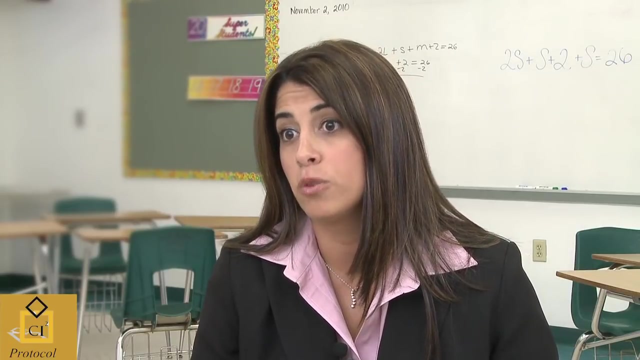 So my main focus, my lesson objective, was to teach them how to translate words into algebraic expressions. So one group had a very clear understanding of how to do that, So I went ahead and worked off them. I brought the students up to the board and allowed them the opportunity, though, to explain their methods. 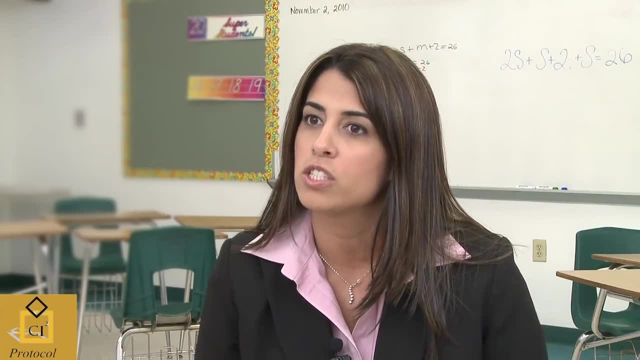 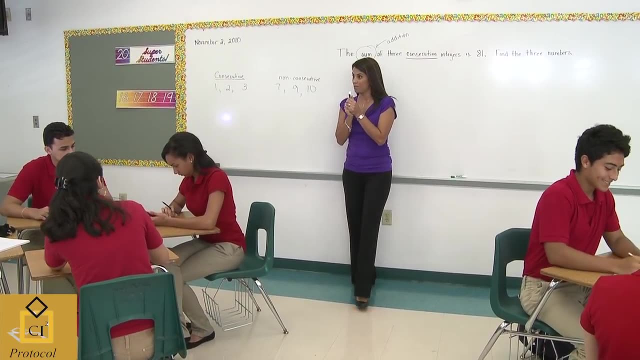 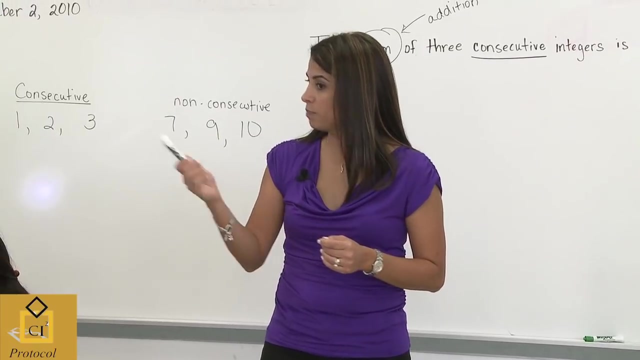 I wanted to show them that there's definitely many different ways to answer a problem And for them to share their perspective on the problem. The ways you got these problems, Believe it or not, every single group did it a little different. Okay, So I'm going to start over here. Please pick somebody to represent your group. 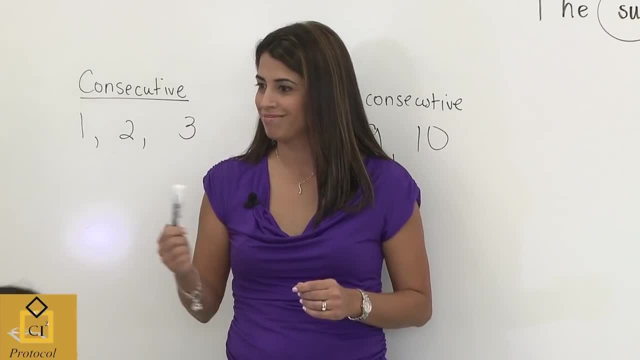 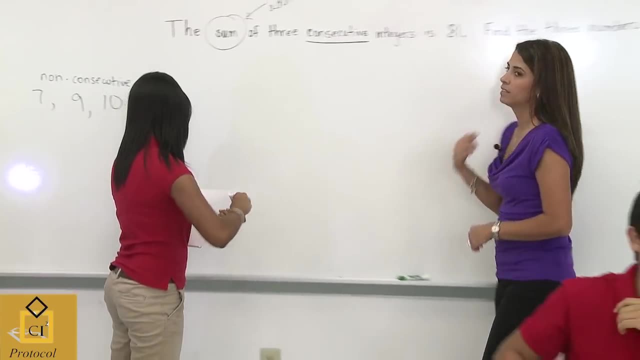 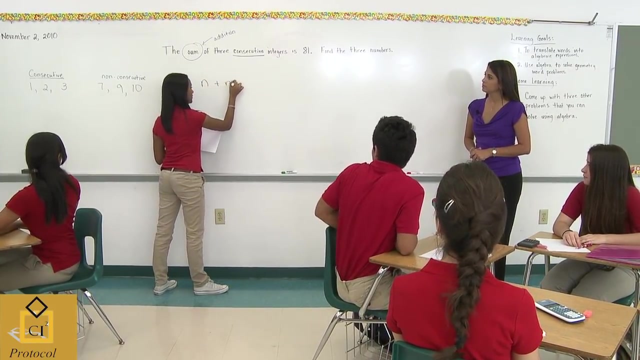 And come on up to show me. Alright, Chris, now it's you. I got the answer because it's saying numbers, so I use a variable. It's n plus n plus 1 plus n plus 2.. Because you're finding three different numbers. 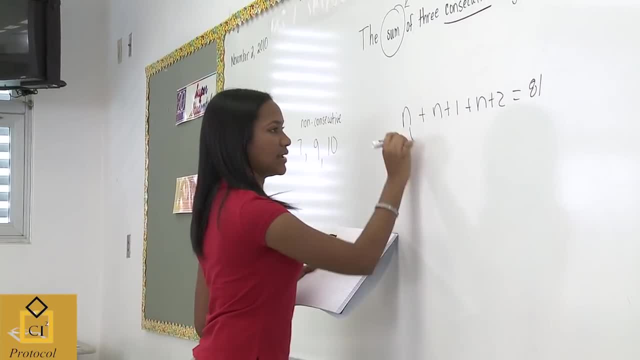 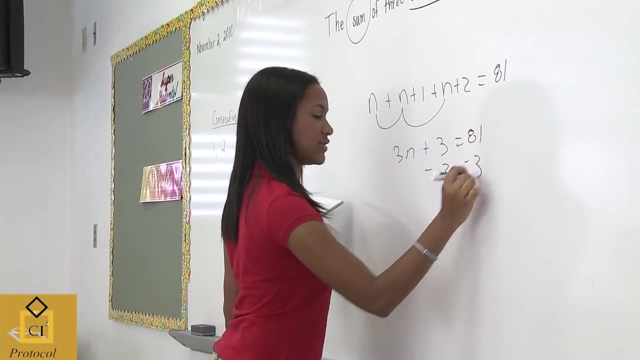 And that equals 81. So I combine like terms. It's 3n plus 3 equals 81.. Minus 3, minus 3.. It's 3n equals 79. Divided by 3.. Divided by 3.. 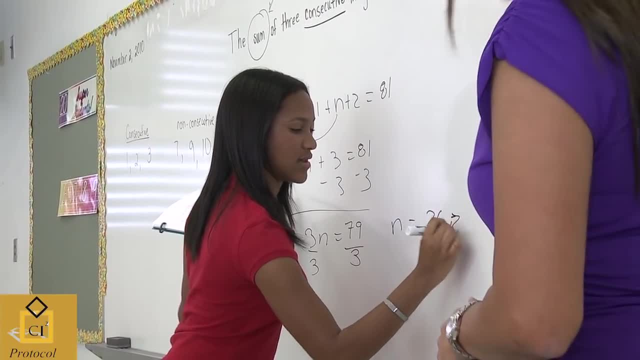 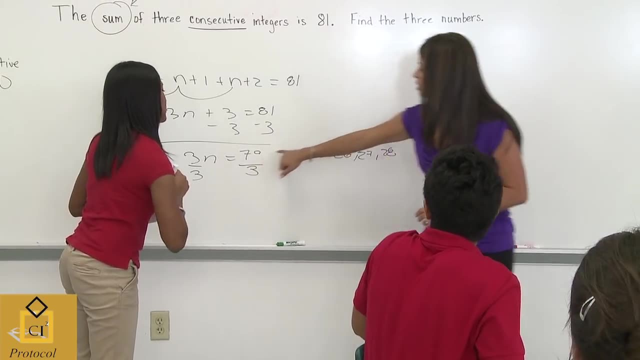 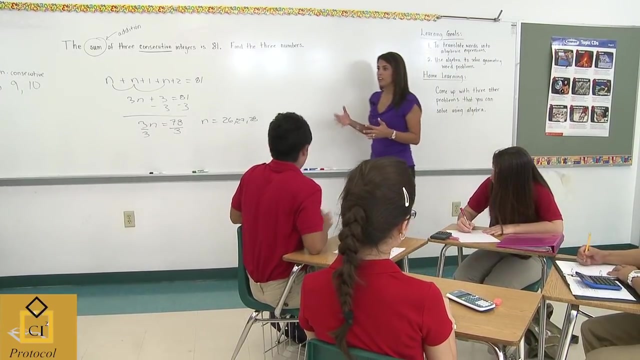 N equals 26,, 27, and 28.. Okay, Sounds good. Put an 8 right there. Put an 8.. Yeah, you got it right. Excellent, Great job, Nice, Okay. so you guys decided to use a variable. 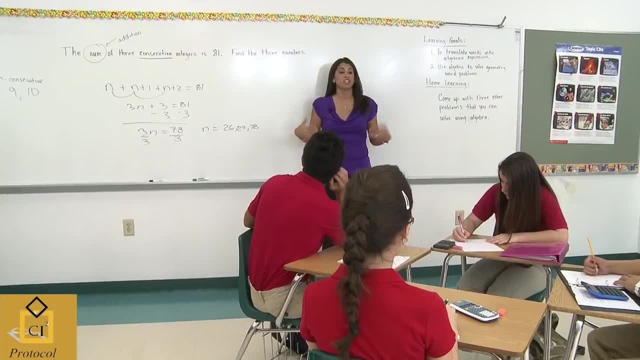 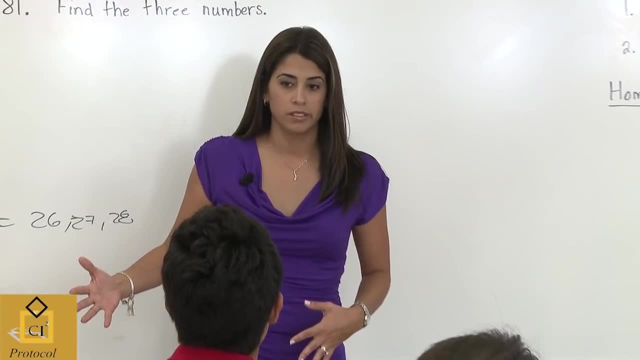 You chose n as your variable. Can you choose any letter? Yes, You could. Can you use a capital letter? Yeah, Yeah, You can use whatever it is. You can use whatever letter you want. Okay, Sounds good. Sounds good. 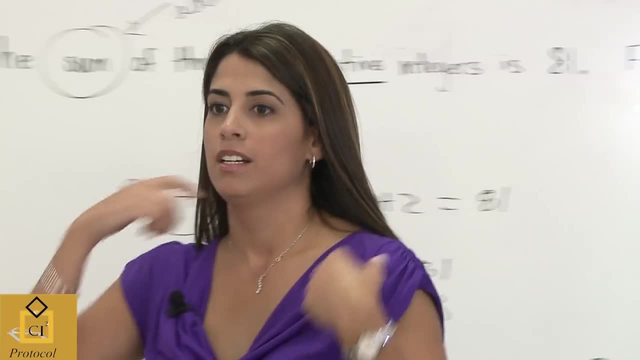 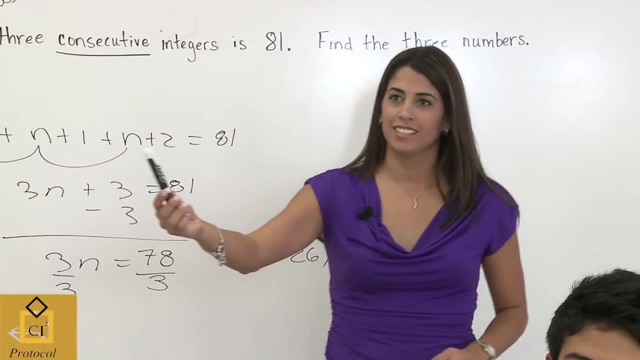 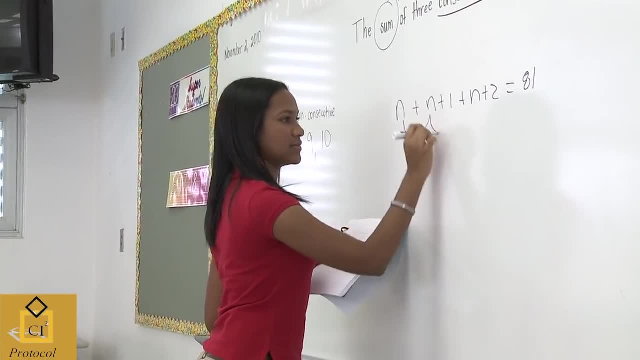 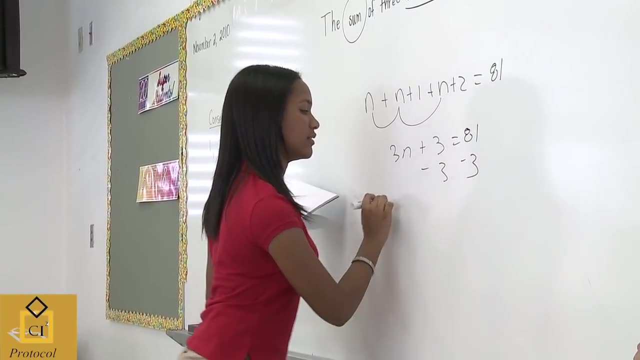 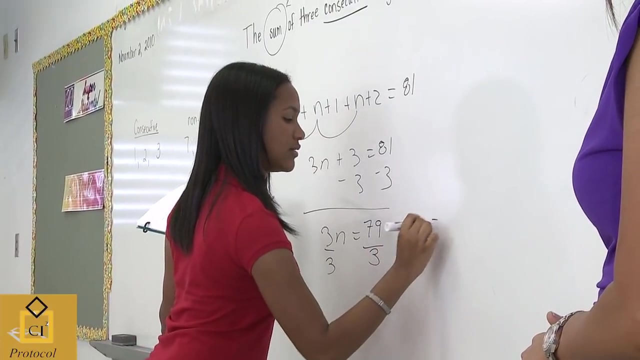 And that equals 81. So I combine like terms: It's 3n plus 3 equals 81, minus 3 minus 3, it's 3n equals 79, divided by 3, divided by 3.. 3n equals 26,, 27, and 28.. 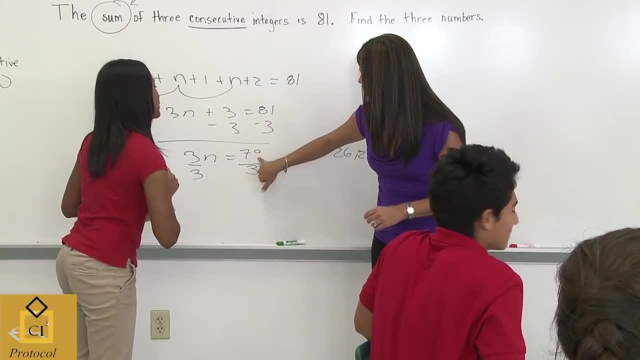 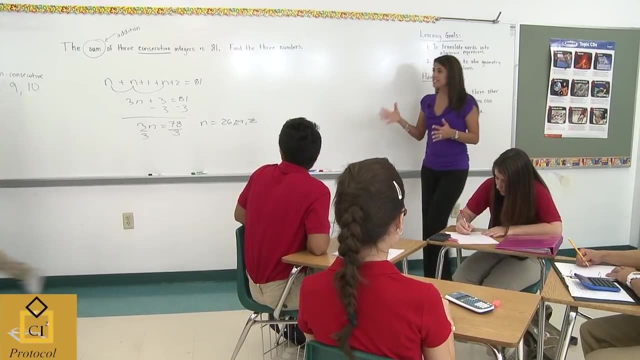 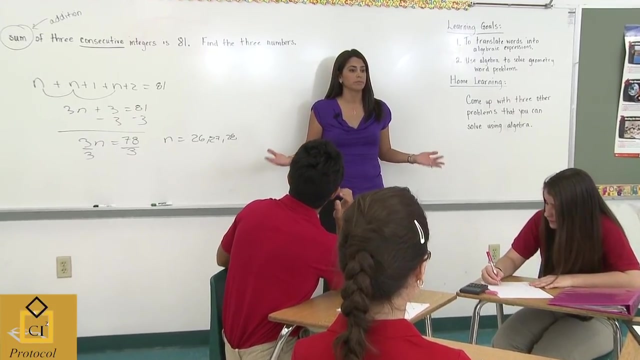 Okay, sounds good. Put an 8 right there. Put an 8.. Yeah, you got it right. Excellent, Great job, Nice. Okay, so you guys decided to use a variable. You chose n as your variable. Can you choose any letter? 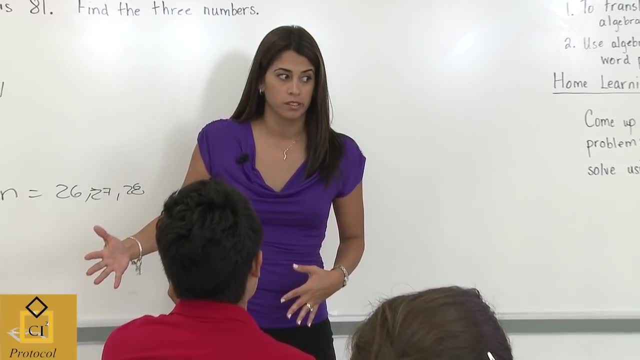 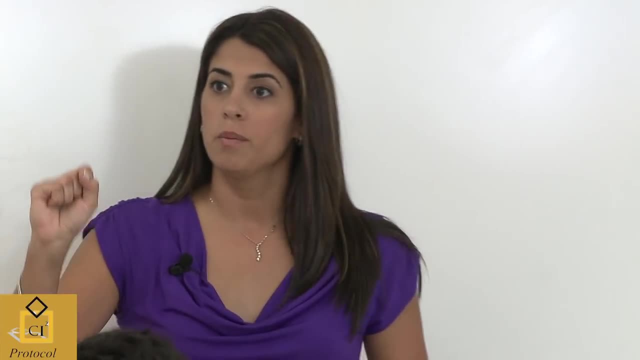 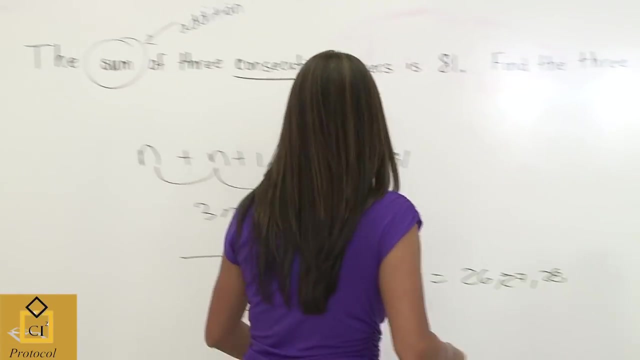 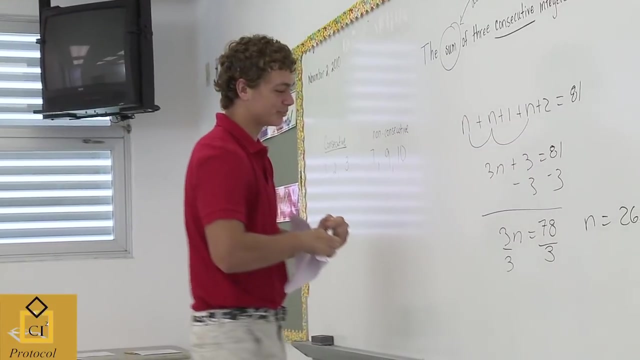 You could. Can you use a capital letter? Yeah, Whatever letter you want. Okay, sounds good, sounds good. Now that group over there pick a representative, please. All right, Chris, come on up. I did it the simple way. 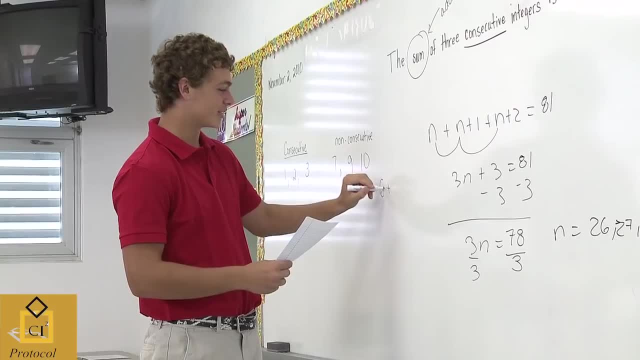 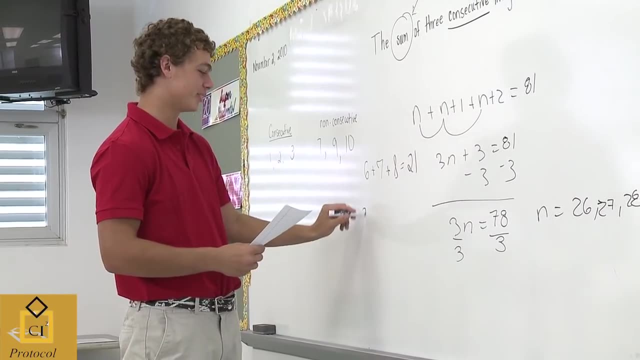 Okay, I just found three numbers that when you add them together they give you something that ends with a 1.. So then I figured you'd have to do 26,, 27, and 28.. Wow, that's extremely interesting. 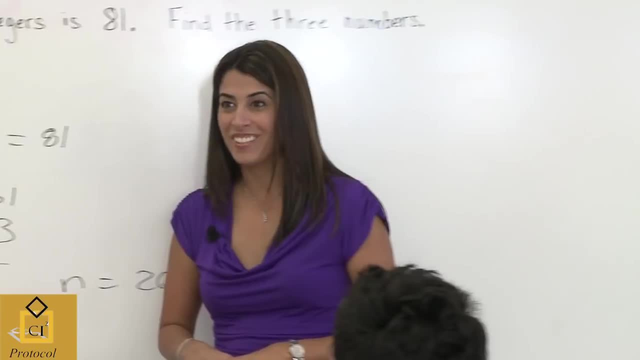 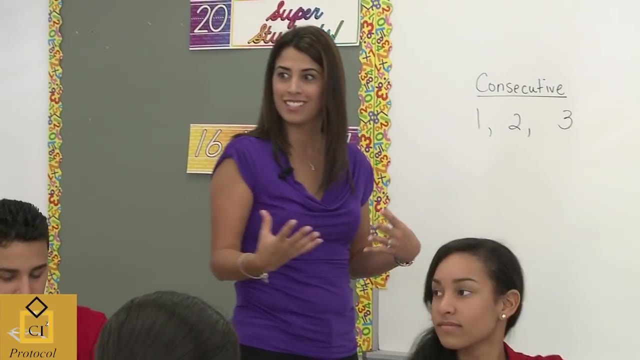 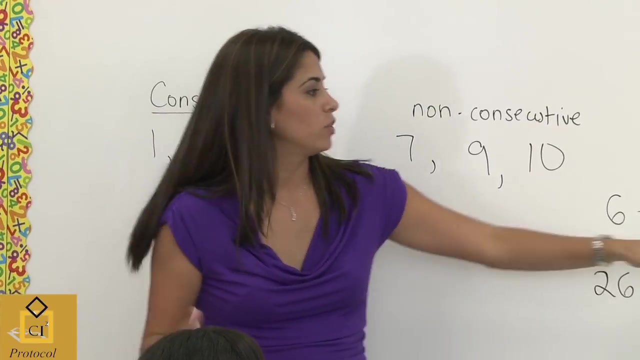 Yeah, Okay, isn't that completely different than what sometimes we think? So it's really important to value everyone else's strategy. He said he thought I need to pick the three numbers, just like you said that would end with a 1 at the end. 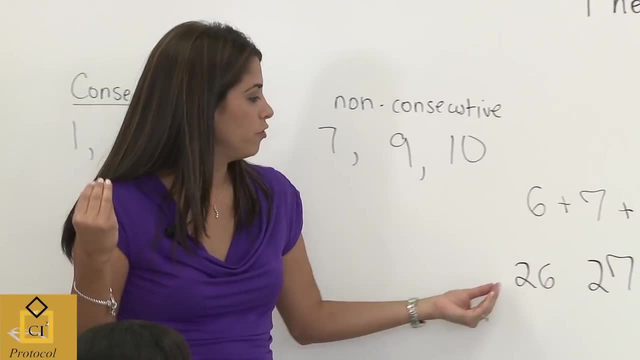 And then, I guess, how'd you end up? how did you figure out a number? I guess? how'd you end up? how did you figure out it was in the 20s? Well, because 8 divided by 4 is 2.. 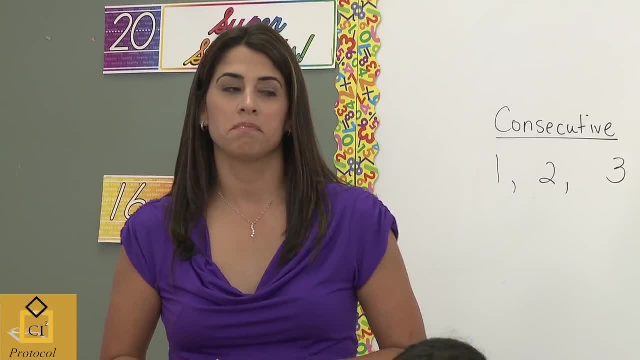 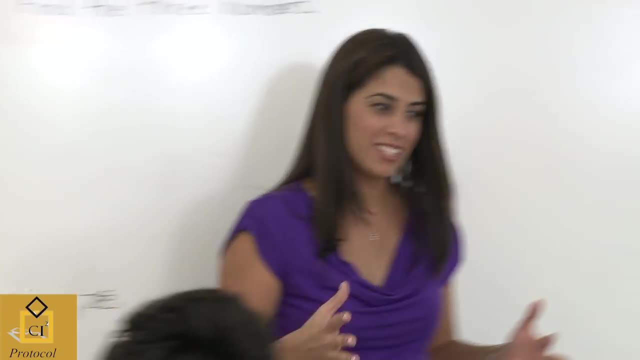 So then, well, 8 divided by 4 is 2.. Okay, So then they all have to be 2s. Very nice method, nice Okay. and then over here, I mean it's perfect the way all of you think so differently. 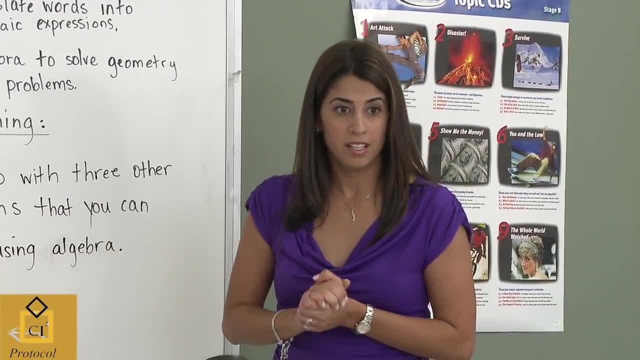 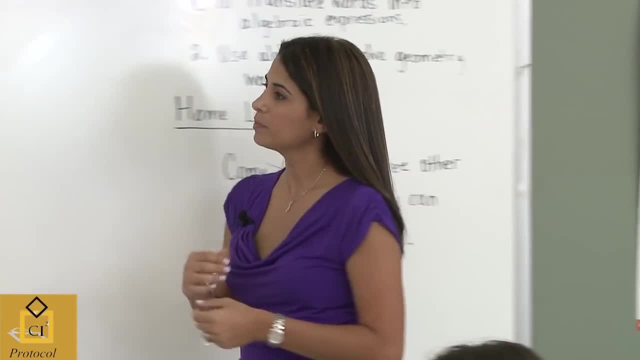 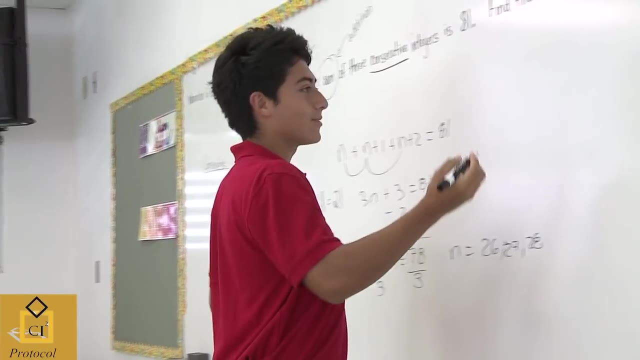 Ernesto, would you like to try it out? Oh, I already got the right one, It was mine, It was Hector. Hector, you want Hector to be the rep for the group? Come on up, Hector. We did it like we told that we couldn't use over the 30s, because if we use three numbers of 30, it's 90,, so it's over the answer. 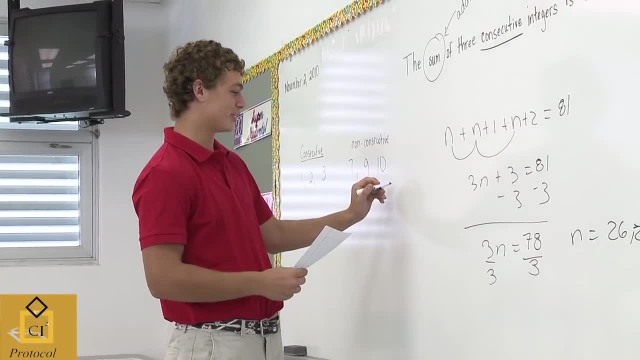 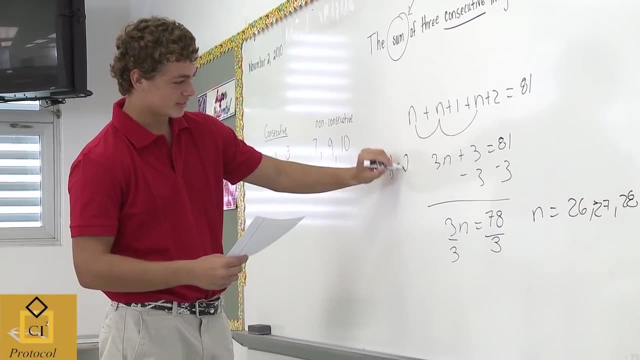 I did it the simple way. I just found three numbers that when you add them together they give you something that ends with a 1. they give you something that ends with a 1.. So then I figured you'd have to do 26,. 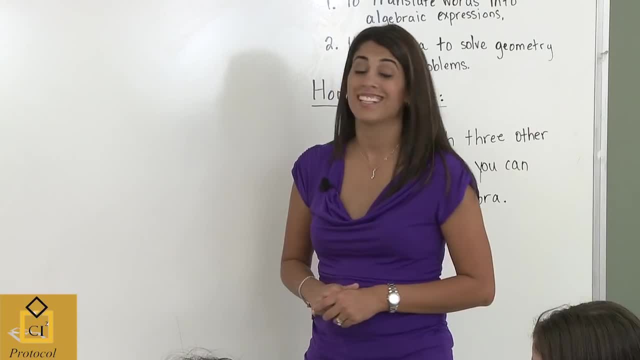 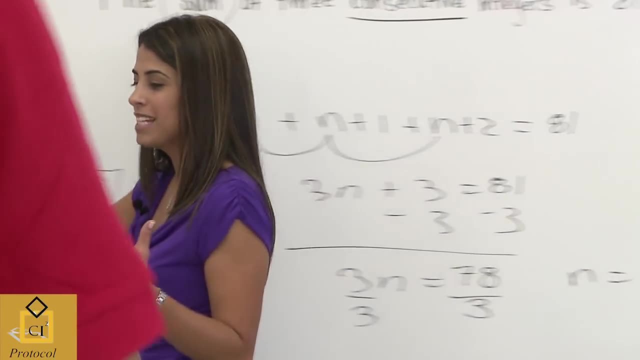 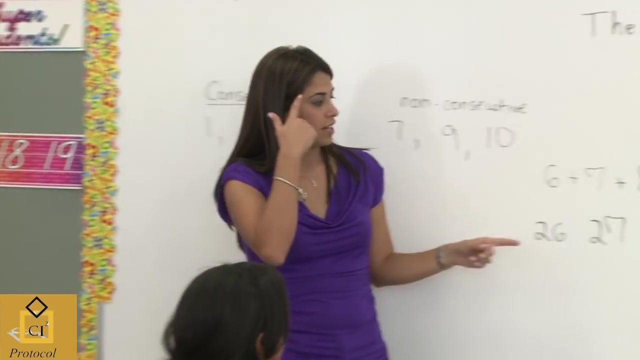 27, and 28.. Oh, that's extremely interesting. Okay, isn't that completely different than what sometimes we think? So it's really important to value everyone else's strategy. He said he thought I need to pick the three numbers, just like. 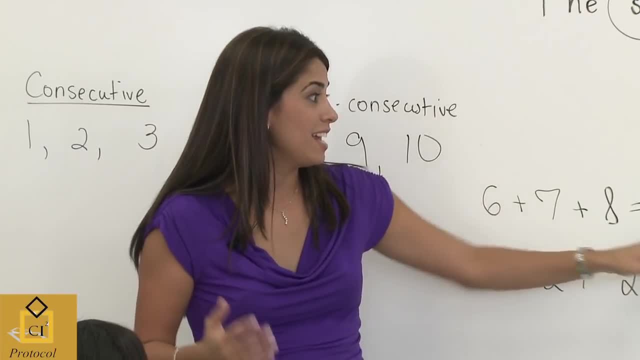 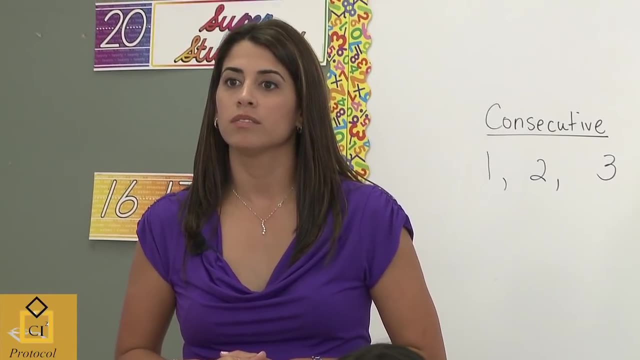 he said that would end with a 1 at the end. And then I guess, how'd you end up? how did you figure out? it was in the 20s. Well, because 8 divided by 4 is 2.. 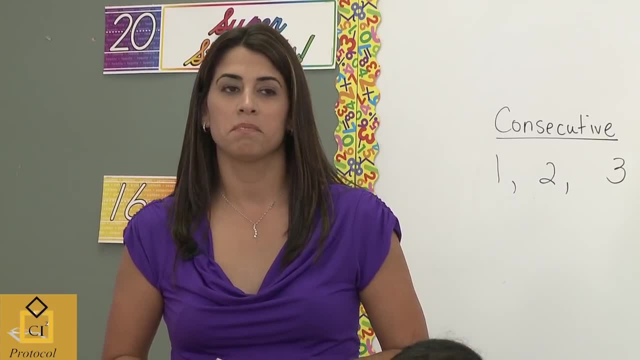 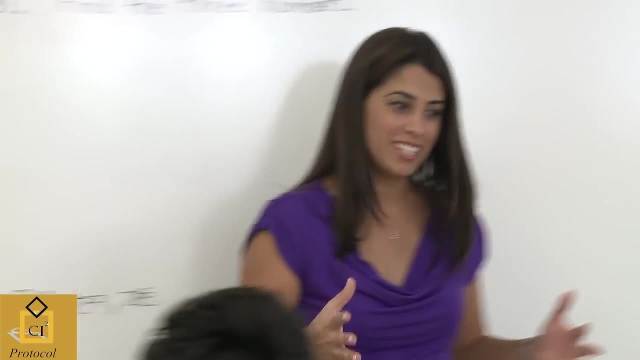 Well, 8 divided by 4 is 2.. So they all have to be 2s. Very nice method, Nice, Okay. and then over here, I mean it's perfect the way all of you think so differently. 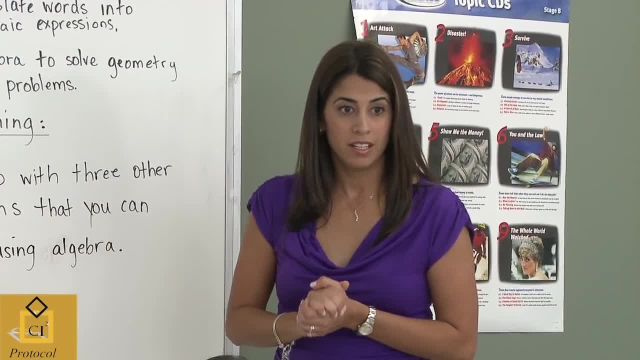 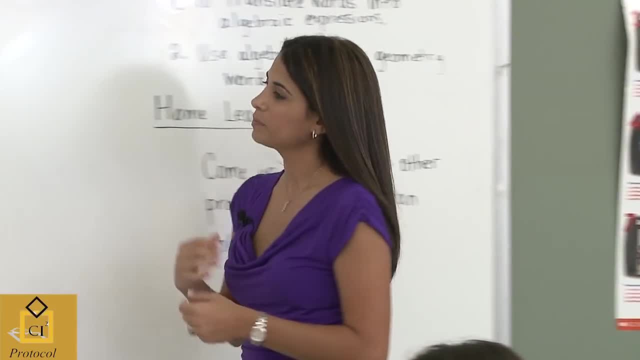 Ernesto, would you like to try it out? Oh, I already got the right one, It was mine, It was Hector. Hector, you want Hector to be the rep for the group? Come on up, Hector. We did it like. 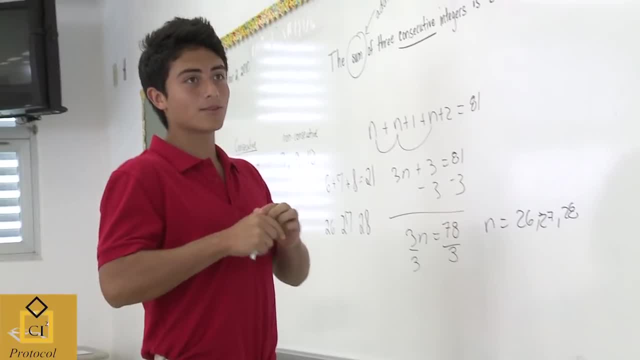 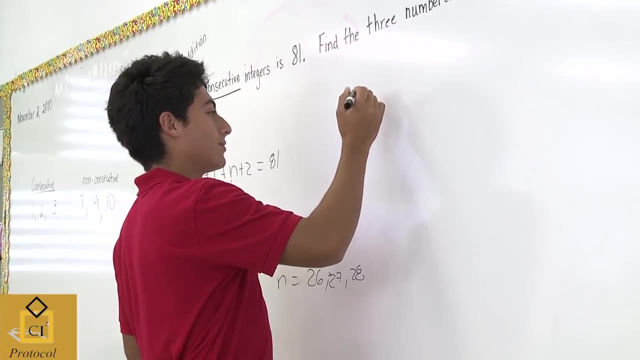 we told that we couldn't use over the 30s, because if we use three numbers of 30, it's 90. So it's over the answer. So it should be between the 20s and the 30s. So we tried out first. 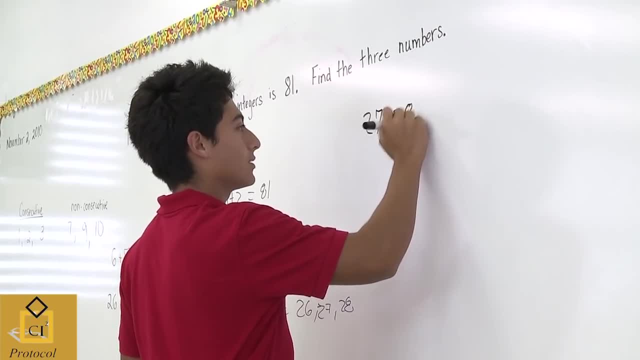 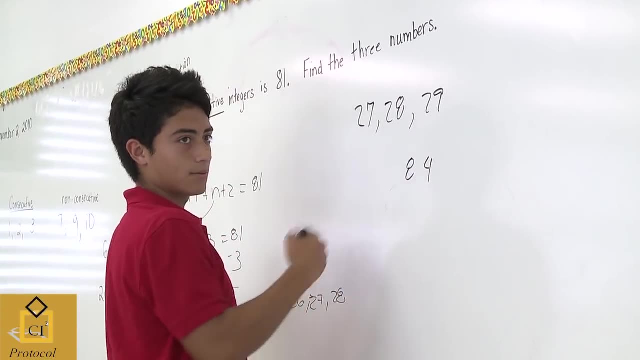 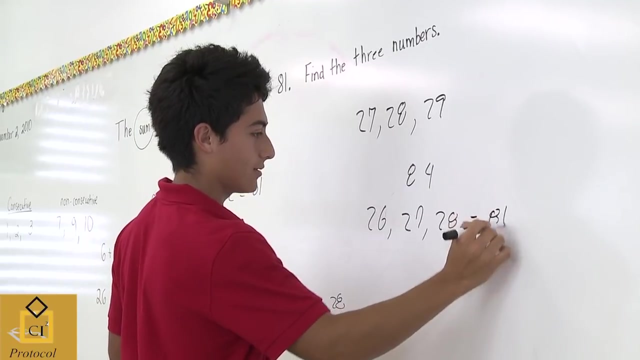 27,, 28, and 29.. And it gave us, I believe it was 84.. So the next few numbers was 26,, 27, and 28.. Okay, And that's the answer. That's the answer. They did it by. 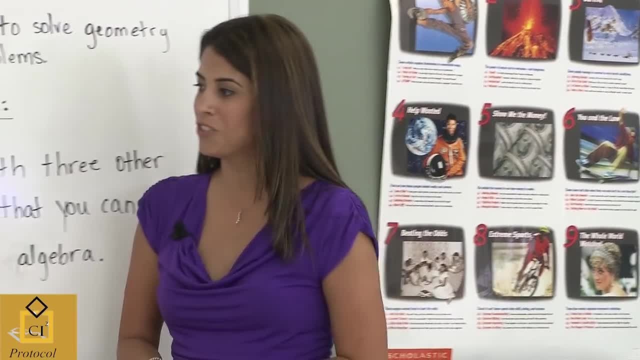 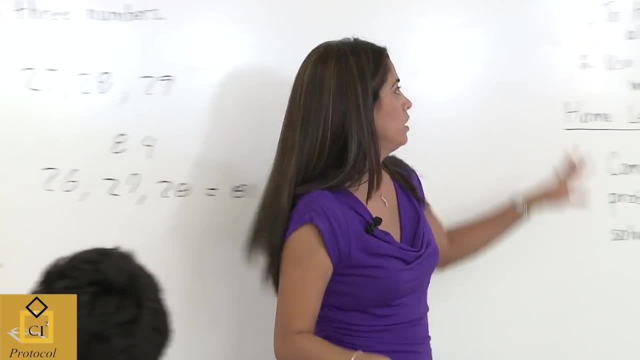 trial and error. Okay, Three different methods, three different strategies, We still got the same number. Now I'm going to focus on the algebraic way, because today we're going to learn how to translate words into algebraic expressions. You did a fantastic job, Bill. 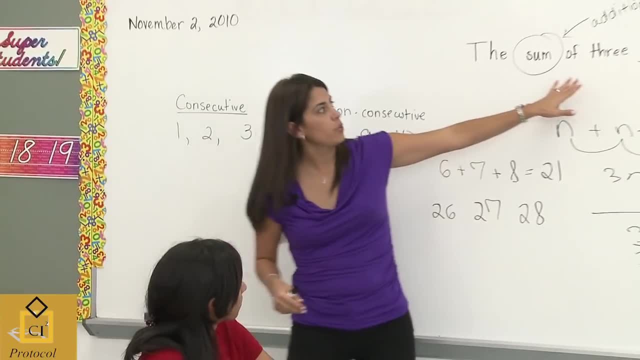 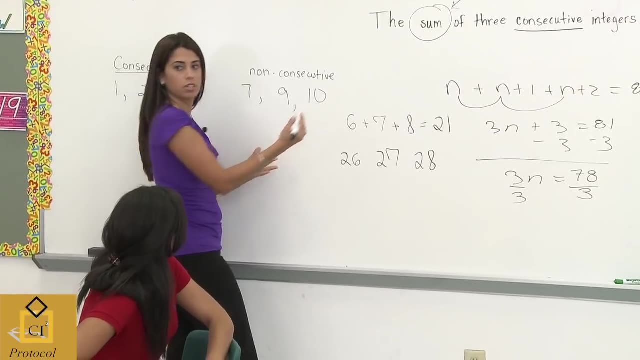 Okay, Now I want you to look here. If we're talking about three consecutive integers, sometimes it would be great to split up those integers. Maybe say number one, number two, number three. Do you think that's a good method? 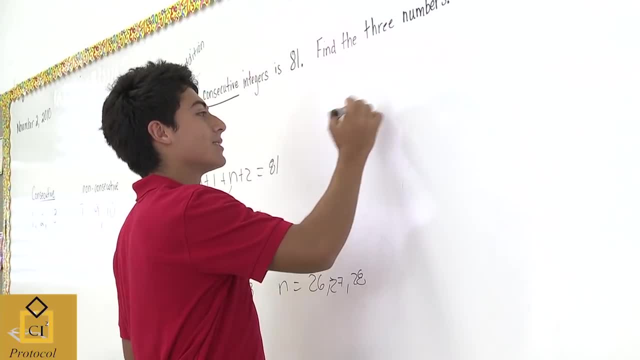 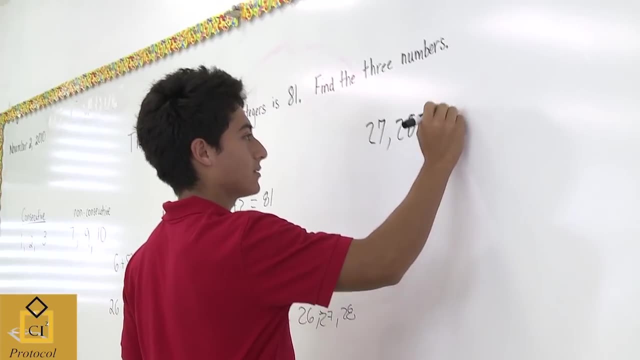 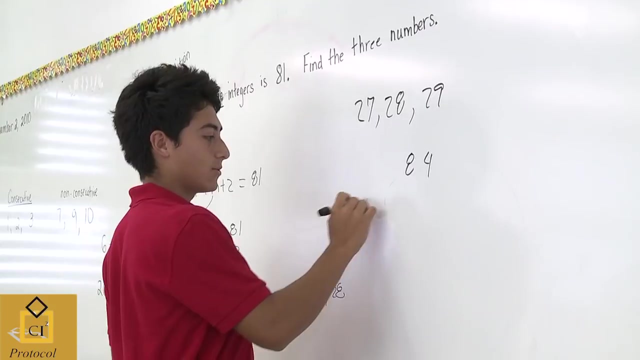 So it should be between the 20s and the 30s. So we tried out first 27,, 28, and 29,, and it gave us, I believe it was 84.. So the next few numbers was 26,, 27, and 28.. 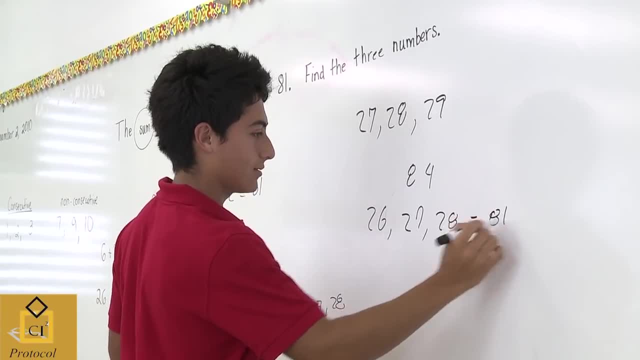 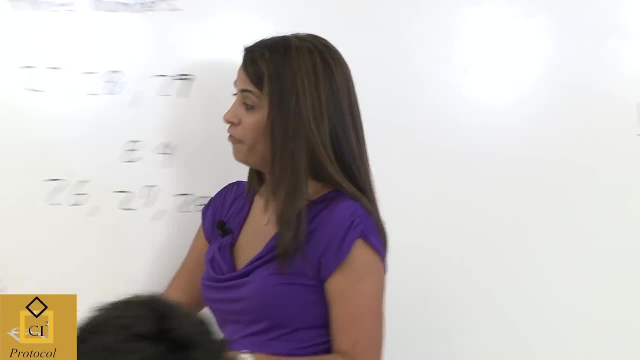 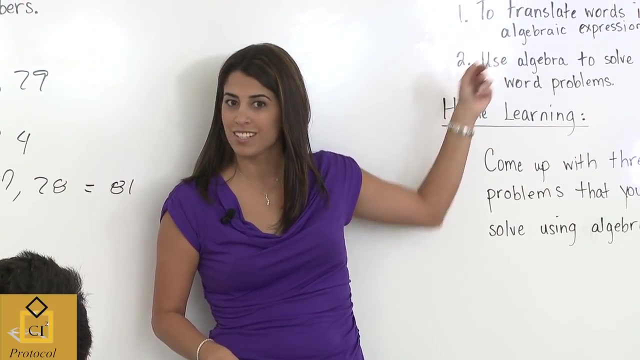 Okay, Nice answer. They did it by trial and error. Okay, Three different methods, three different strategies, we still got the same number. Now I'm going to focus on the algebraic way, because today we're going to learn how to translate words into algebraic expressions. 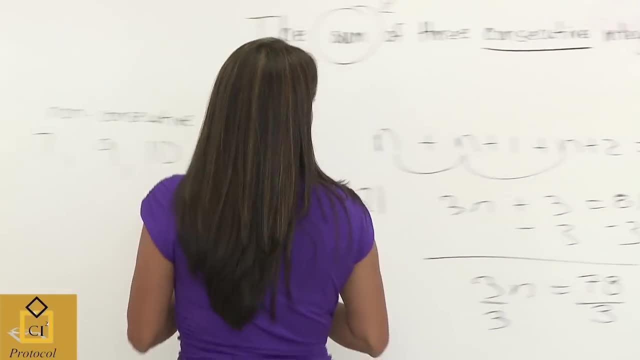 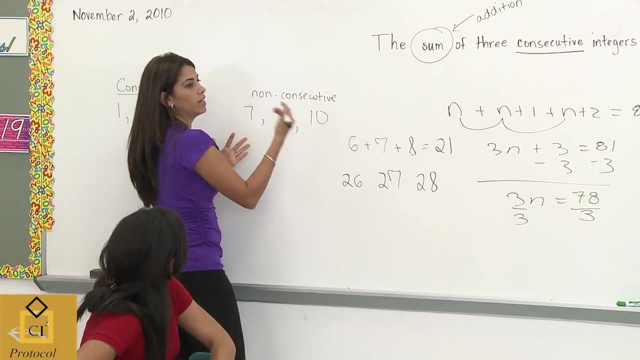 You did a fantastic job, Bill. Okay, Now I want you to look here. If we're talking about three consecutive integers, sometimes it would be great to split up those integers. Maybe say Number one, number two, number three. 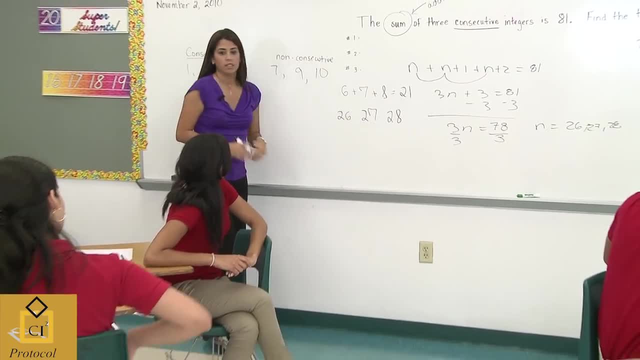 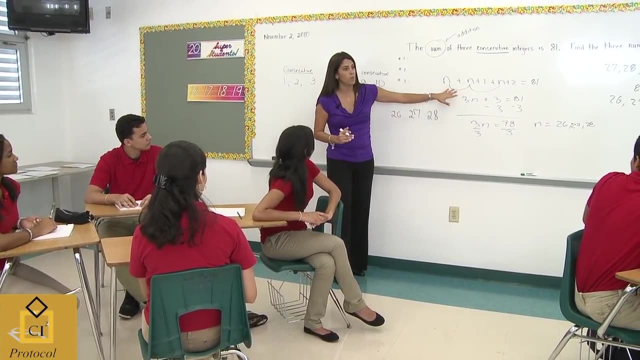 Do you think that's a good method? Do you like that? Do you like listing it? No, you don't. Okay, So how about we just then, by looking at this problem, how about we kind of break them up? Do you like that? 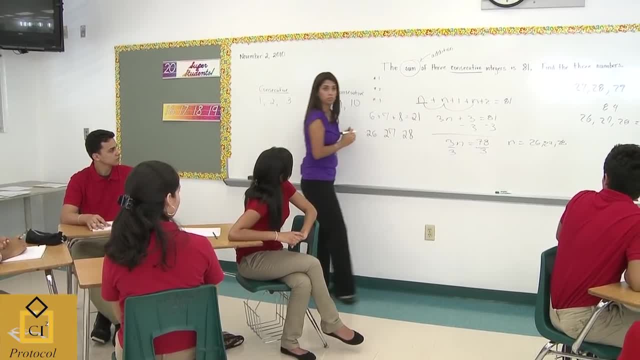 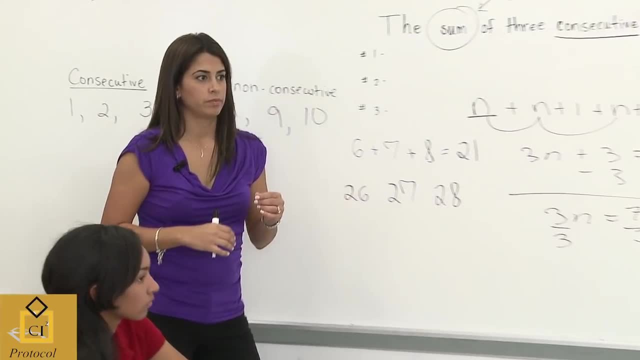 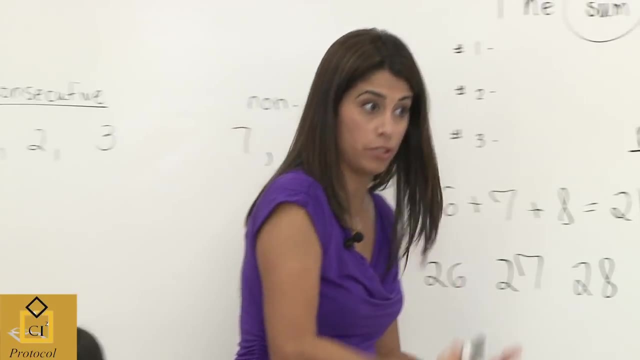 Yeah, Okay, So we'll say this is the first one, first integer. Why would the second integer be n plus one? Second consecutive number, Second consecutive number. You did plus one, So it could be consecutive Right plus one. 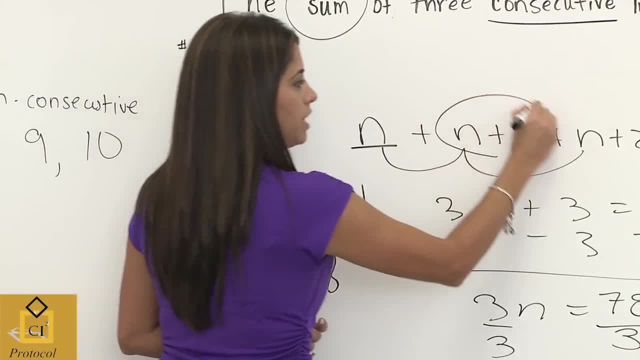 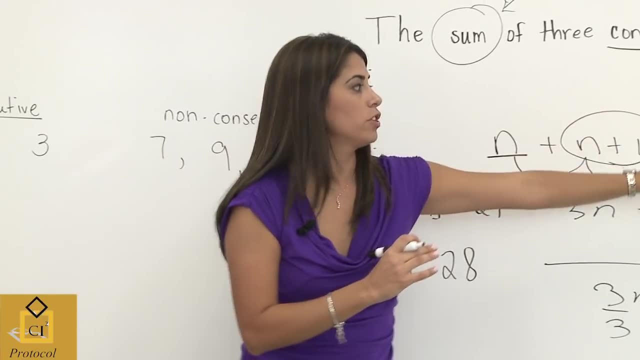 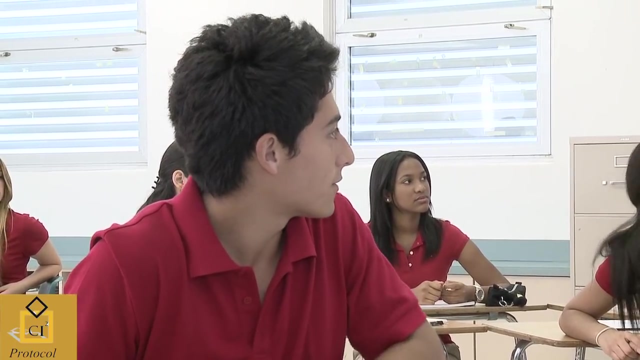 So it's the number you did plus one. Great, So this would be the second consecutive integer. Okay, So you can clearly see one, two. and what's the third one? and why is it n plus two? Because it's the first number you use, plus two after two consecutive numbers. 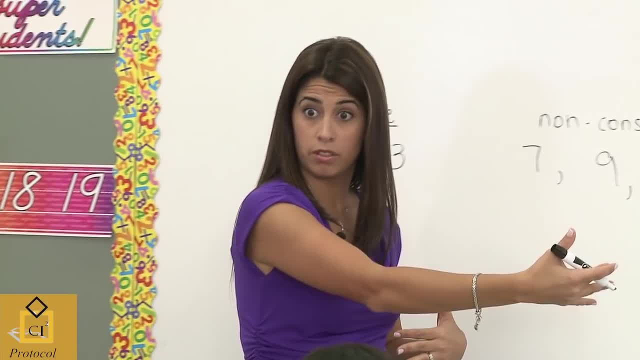 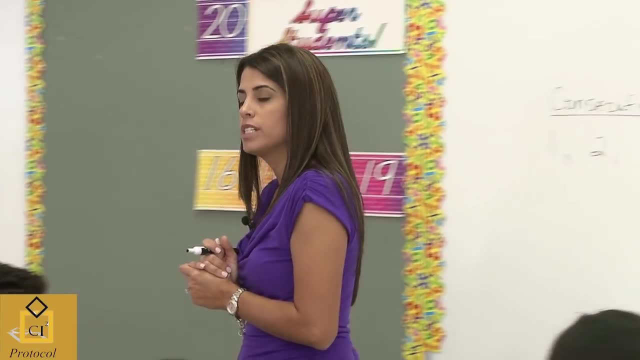 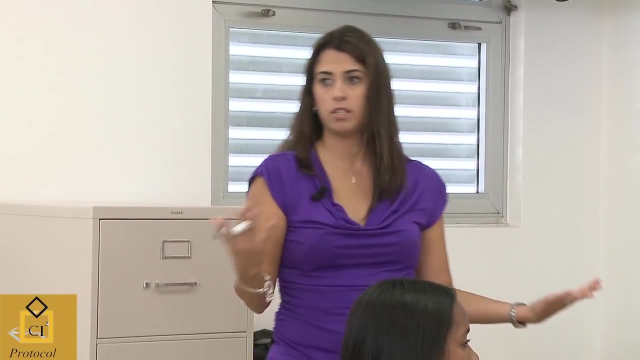 That's right. Plus one is the second number, plus two is the third number. Okay, So it's in between those sets of numbers. What do you notice, Chelsea? That they're adding them together. They're adding them together, And why did you choose to add and not subtract or multiply or divide? 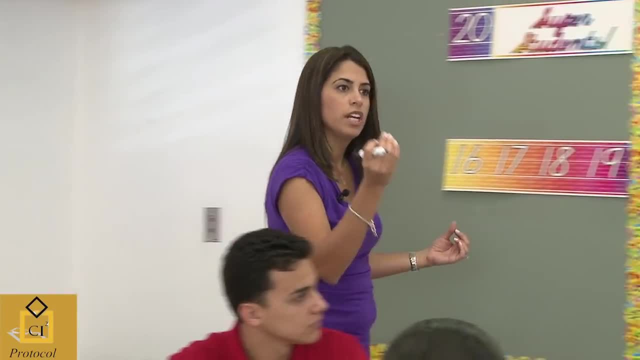 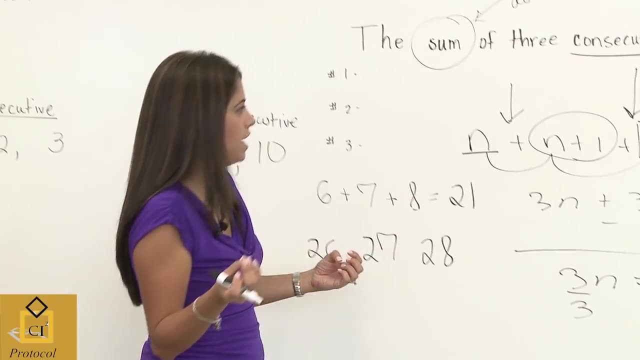 It's easier. It's easier. What key word in the problem gave you to show that method? It was positive, Okay, positive, Nice. And then we want to come up with the same total, a total. the sum So equals eight. 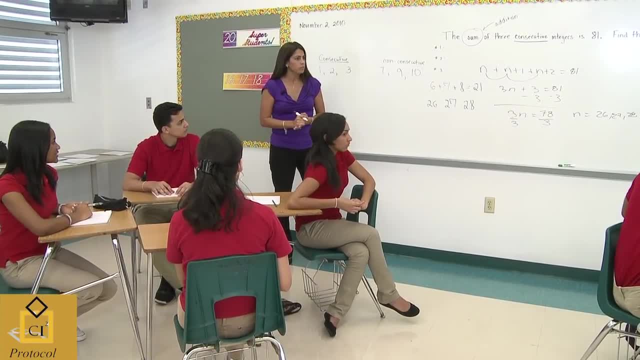 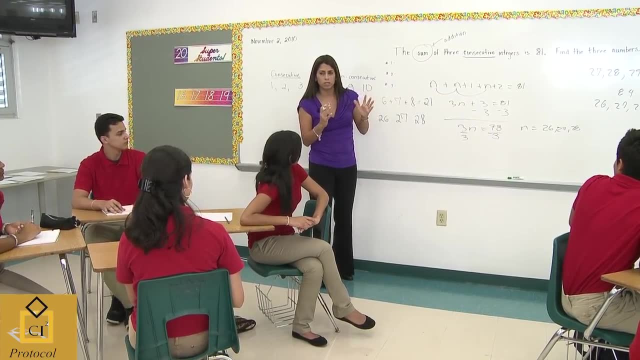 Do you like that? Do you like listing it? No, You don't, Okay. So how about we just then, by looking at this problem, how about we kind of break them up? Do you like that? Yeah, Okay, So we'll say: 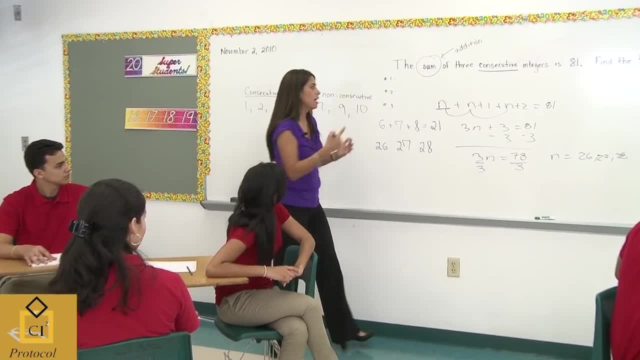 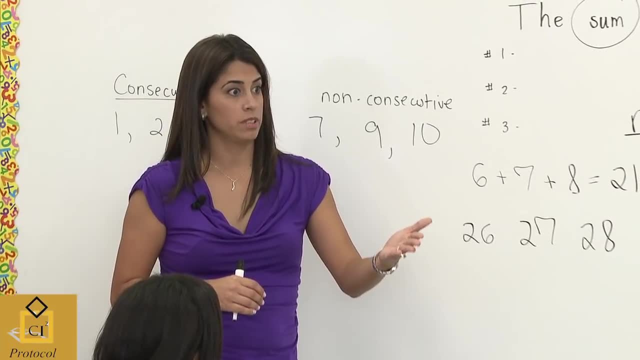 this is the first one, first integer. Why would the second integer be n plus one? It's a consecutive number, So it's the number you did plus one, So it could be consecutive, Right Plus one, So it's the number you did. 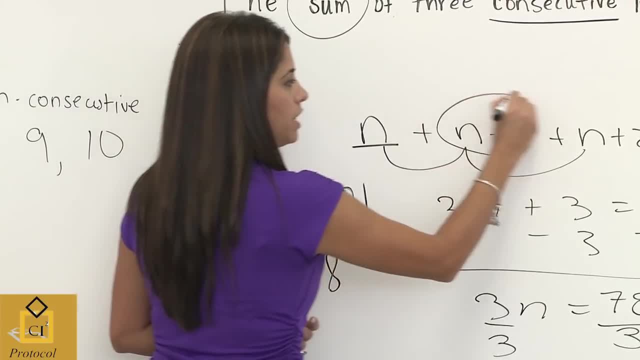 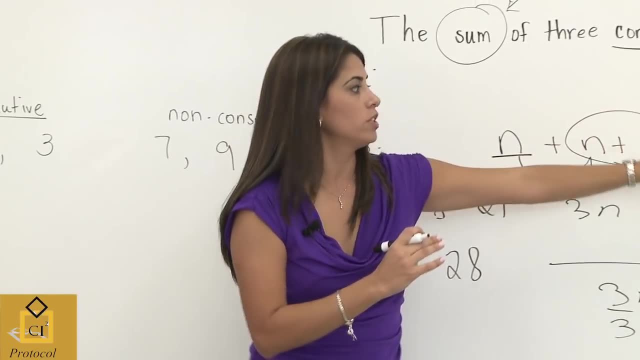 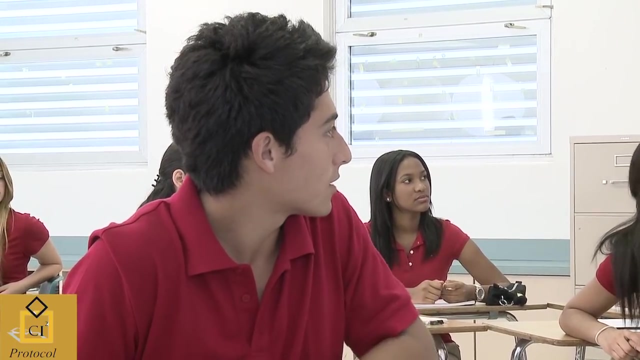 plus one. Great, So this would be the second consecutive integer. Okay, So you can clearly see one, two. and what's the third one? and why is it n plus two? It's the first number you used, plus two, after two consecutive numbers. 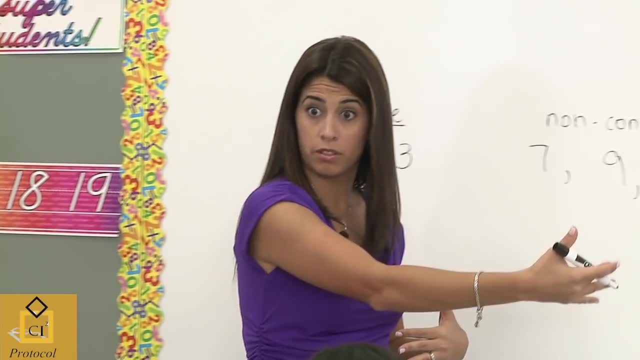 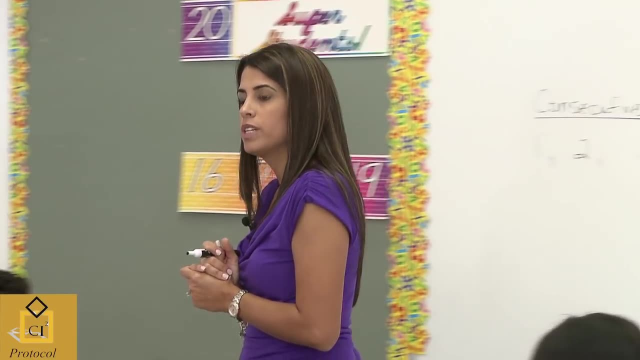 That's right. Plus one is the second number, Plus two is the third number. Okay, What do you notice? that's in between Those sets of numbers. What do you notice, Chelsea? That they're adding them together. They're adding them together, And why did you? 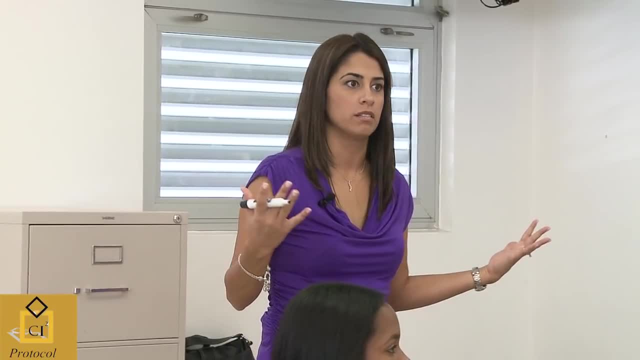 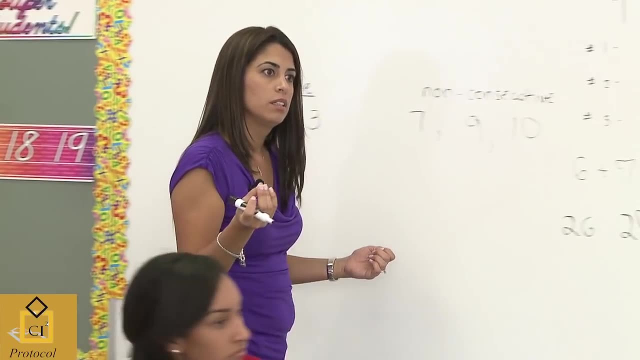 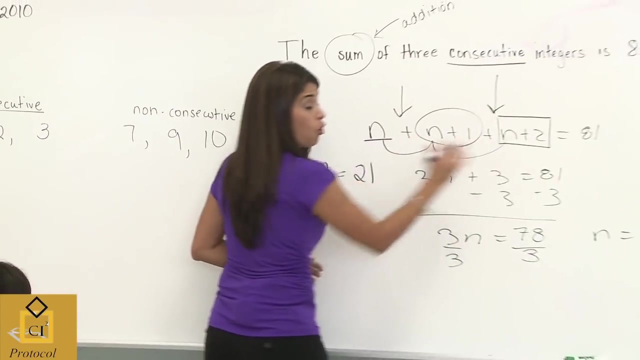 choose to add and not subtract or multiply or divide. It's easier. What key word in the problem gave you to show that method? It was positive, Okay, Positive, Nice. And then we want to come up with the same total, a total. 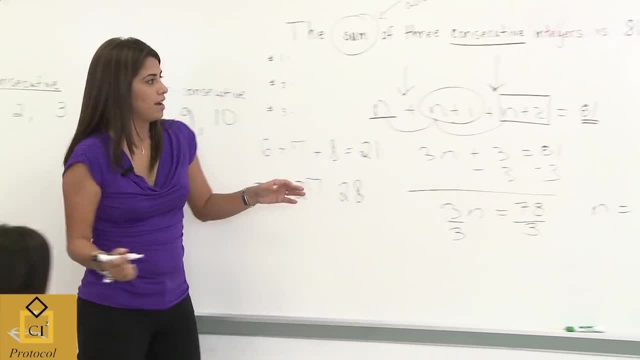 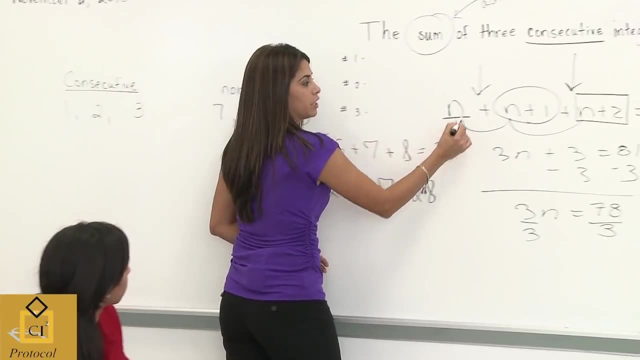 the sum that equals 81.. Now, I like the way, Chris, now that you combine the ends. Okay, It was almost like here's one, here's the other, here's the other. How many ends do you have together? 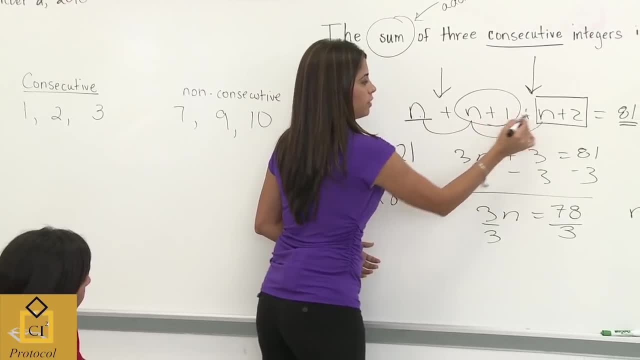 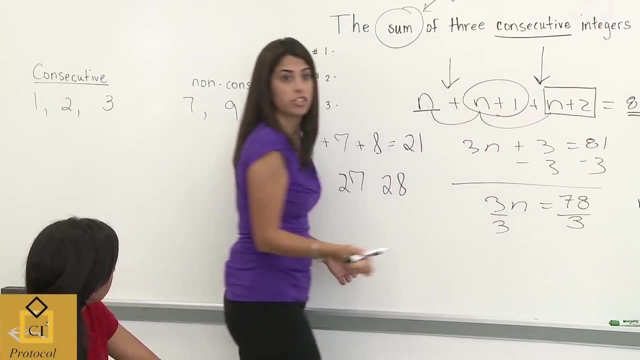 Three. There it is One, two, three. She put little loops to represent it, And then she combined the constants one and two. What's one plus two, Three? Good, And then we solve an equation like we normally do. 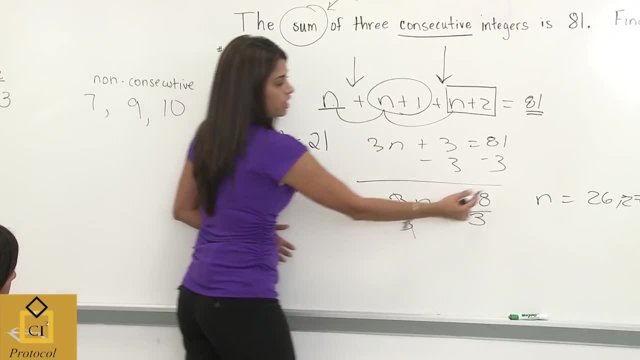 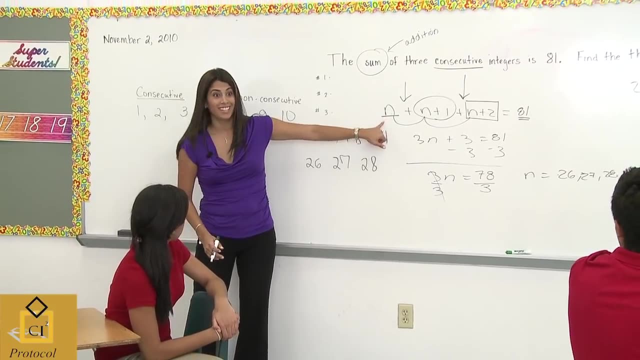 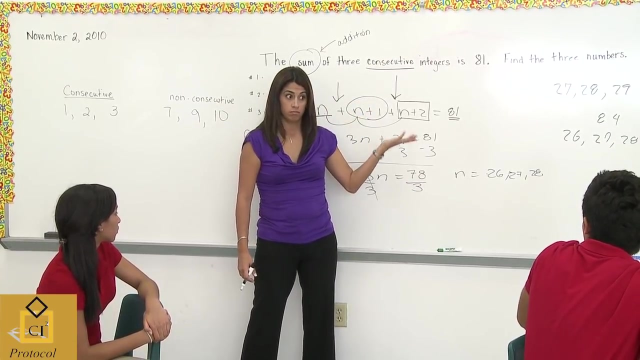 And then, of course, divide by three, She got 26.. Twenty-six represents which one of these End Good, Twenty-seven, So twenty-six plus one. Can I actually substitute this number in to check my answer? Yeah,